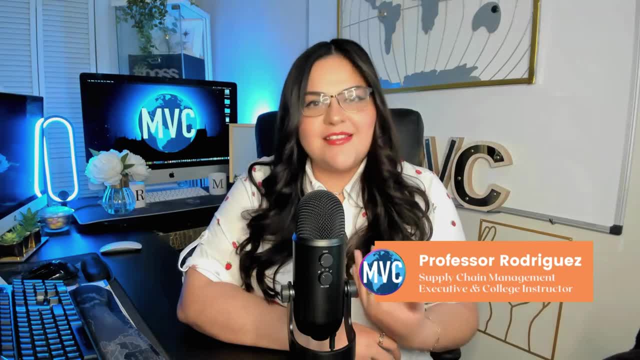 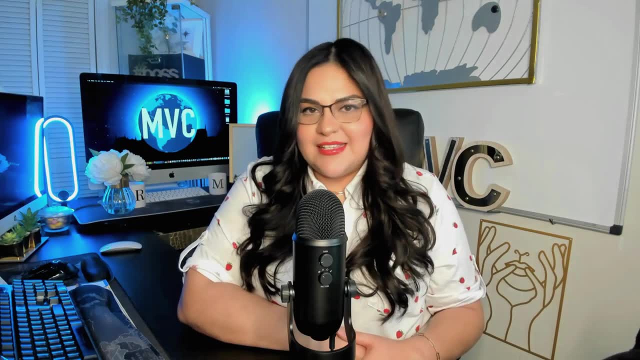 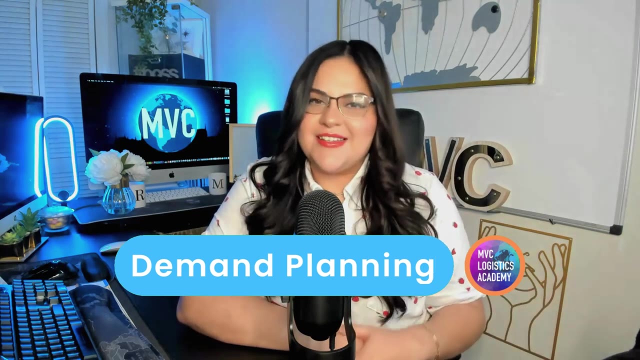 that in a way that's easy to digest, and also I bring you career development advice that's easy to implement. Now, in today's lesson we're going to talk about lesson number eight, and that is demand planning, or what is demand planning? If you've been watching this series, the learning, 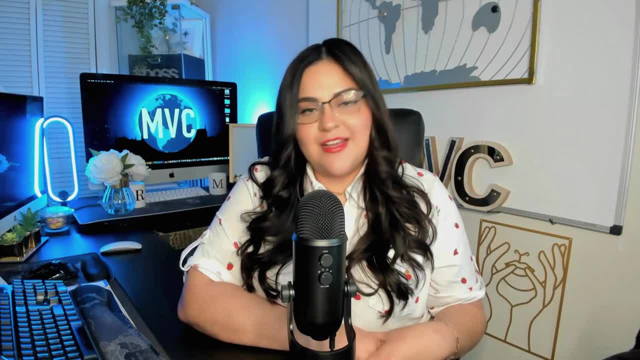 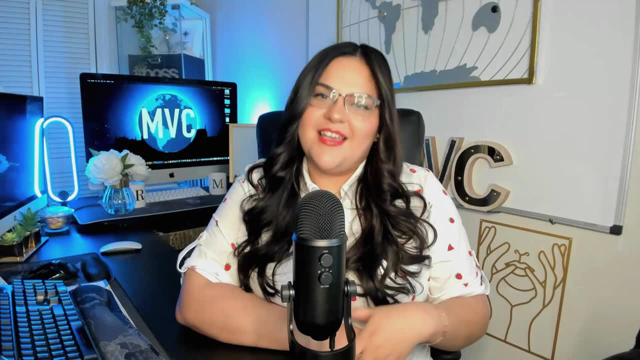 logistics series. you know that we progress on sort of the topics that are building the foundation from what is supply chain and we're building up to those bigger concepts in the area of supply chain management. So that's what we're going to talk about today: demand planning. I. 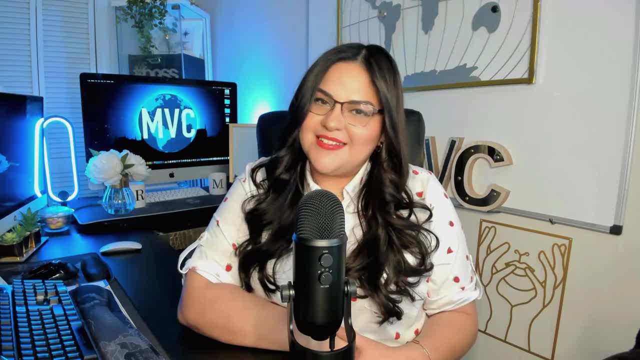 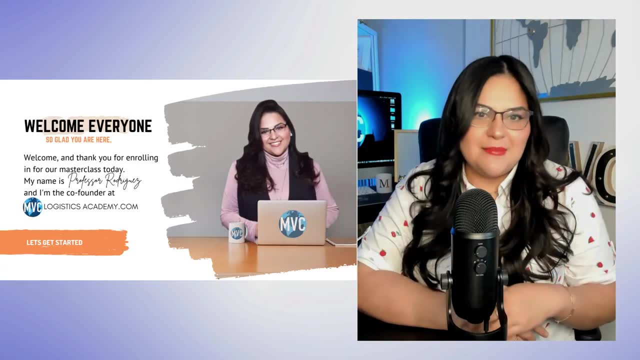 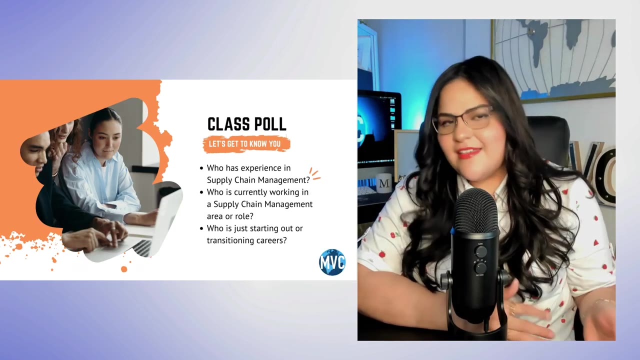 hope you have been watching the videos and I hope you enjoy this one, so let's get right to it. I also want to let you know that I am offering a free master class on supply chain career development, where I help students and professionals like you figure out what their ideal supply chain career can look like and how. 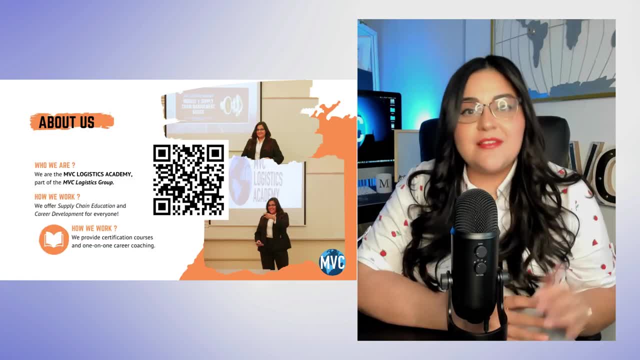 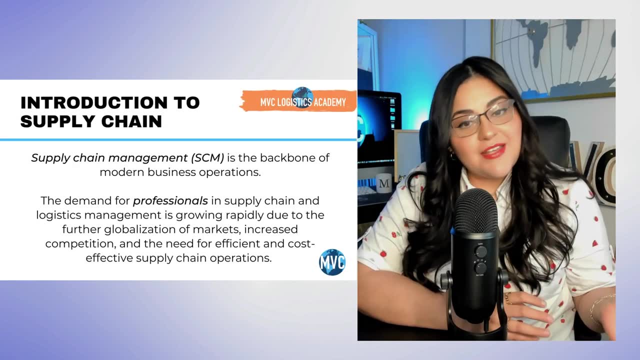 to actually get there. I talk a little bit about what is supply chain management, some sort of the foundations on that, but I do focus more on what are some career paths that you can find in supply chain. what are some of the skills and some of the competencies you'll need for a career in supply? 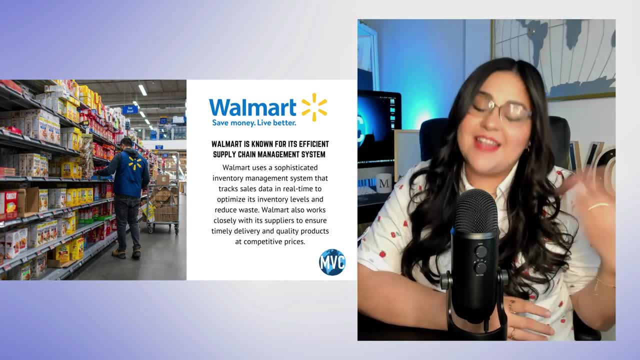 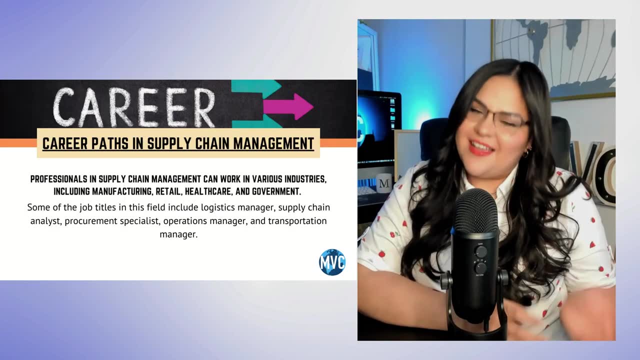 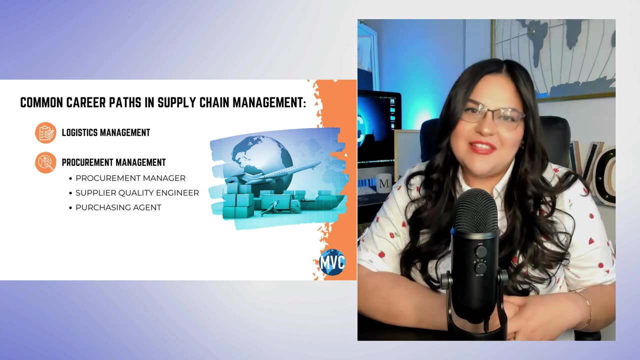 chain and some of the students that have previously taken this class and have been coached by me in that area. In this master class you get to chat one-on-one with me live on a zoom call in one of our supply chain career development master class sessions. I will have all the links in the description. 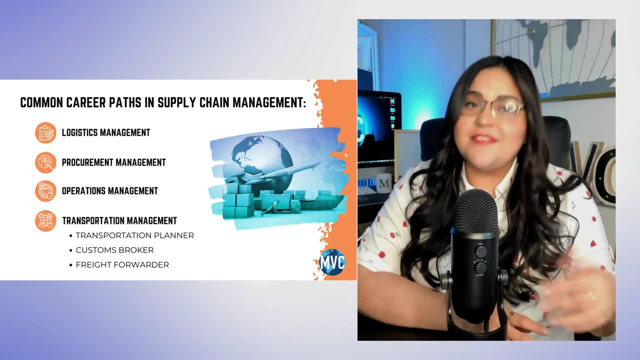 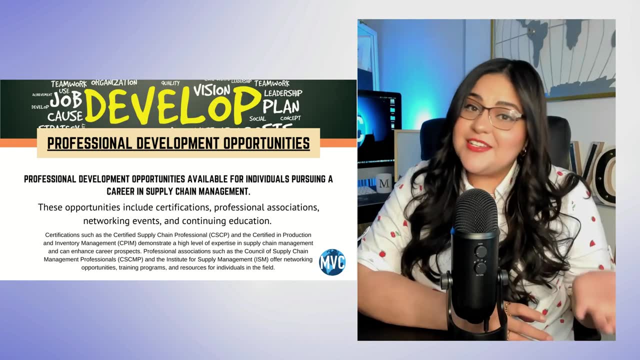 down below with the times and the dates for the upcoming session. We had a lot of great feedback on the last one. I really hope you can join, So if you're interested in that, I'll be happy to help you, And if you have any questions, you can reach out to me on the chat box And I'll be happy to help you with any questions. 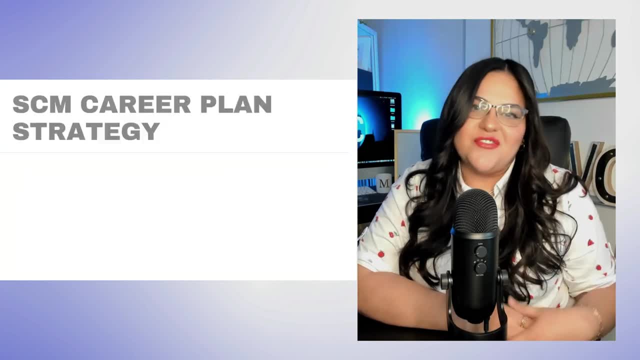 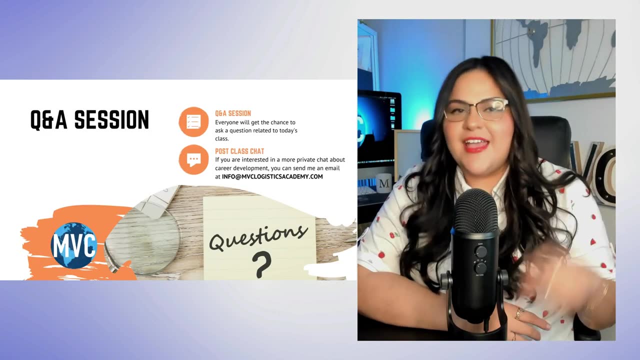 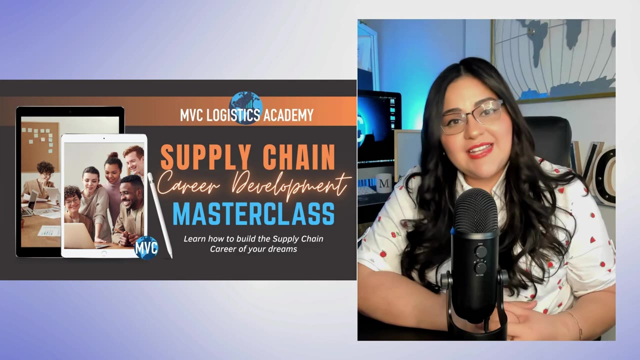 And to chat one-on-one with me in a live zoom call for the master class, then I will put the description and the information and the links down below, And some are here in the cards as well. So we'll try to do that, All right. So without further ado, let's get into lesson number eight, demand. 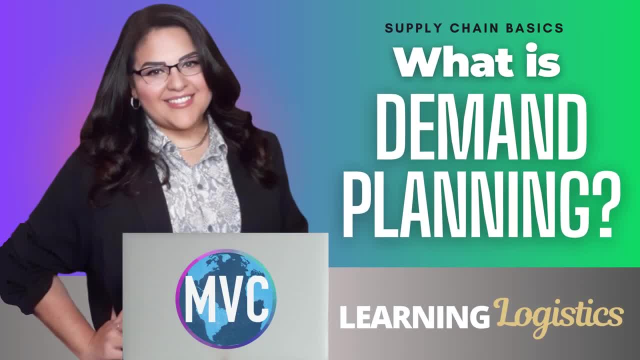 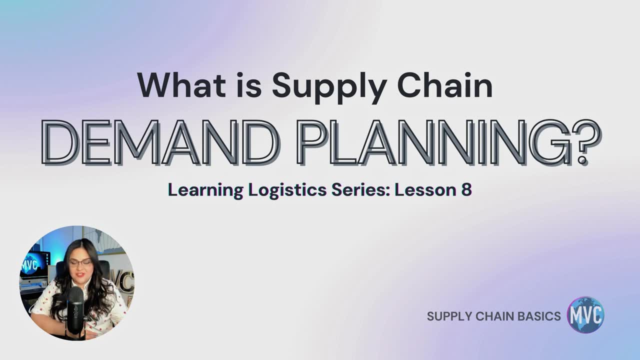 planning. In today's lesson, we're going to focus on demand planning, which is a progression of the topics that we've been talking about within the bigger bubble of supply chain and supply chain management. As I mentioned earlier, I have made a video on demand planning previously, and this was 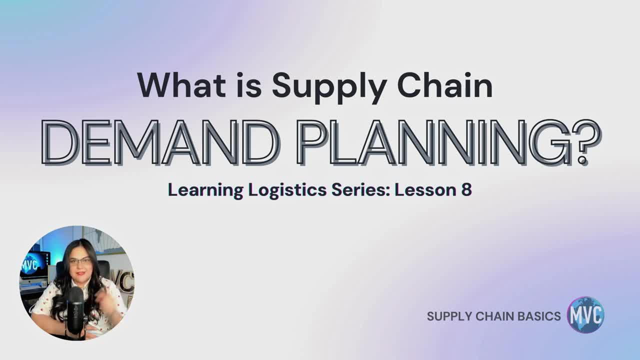 earlier when the channel was getting started, And I'm going to add them in the links, somewhere in the card somewhere And you could always check that video out. But in this video I'm trying to take an approach that is a little bit easier to learn and to understand about what is demand planning. 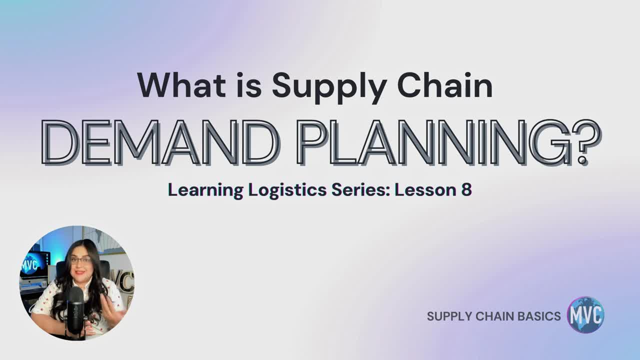 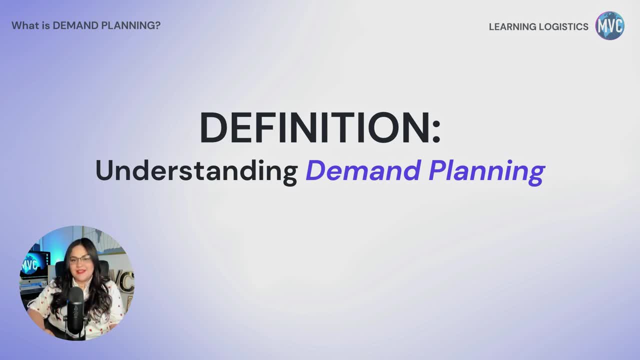 and sort of updated for 2023.. Giving you some examples that apply to today's environment as well. First up, we're going to start with the definition, So we have to understand what is demand planning. Demand planning really is a very crucial. 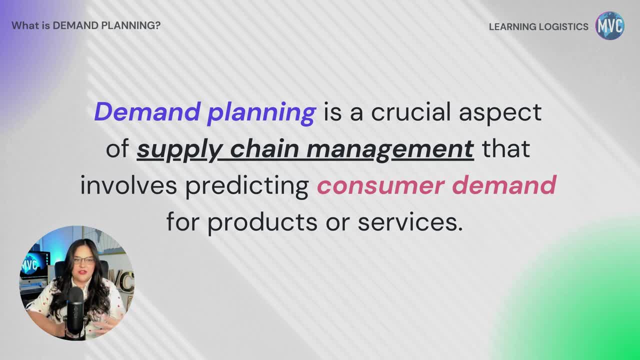 aspect of supply chain management as a bigger picture as a whole And that really within demand planning. what it really involves it's predicting consumer demand for the products and services that our business offers. Now, by accurately forecasting demand, businesses can really optimize their inventory levels. 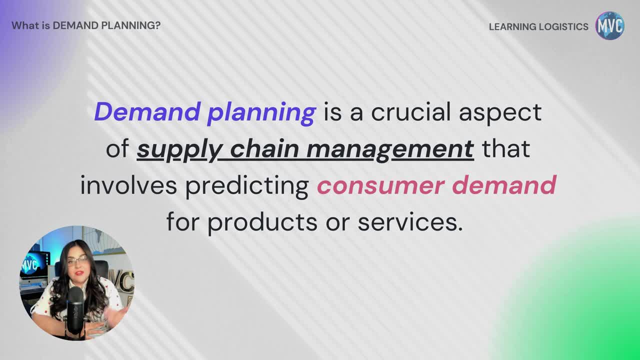 they can reduce waste and they can improve their bottom line when they plan for their demand and their levels of demand. Now, in this lesson, I'm going to take you through what's the importance of demand planning. I'm going to highlight some examples of some companies that have implemented. 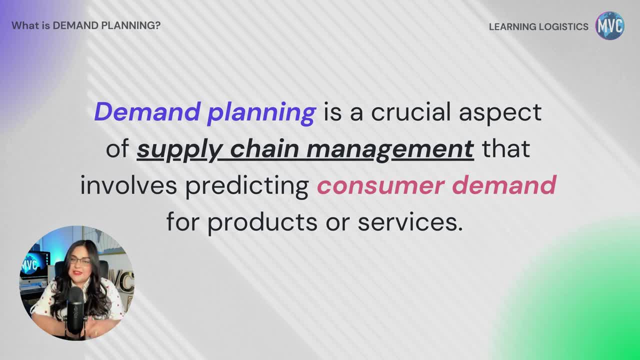 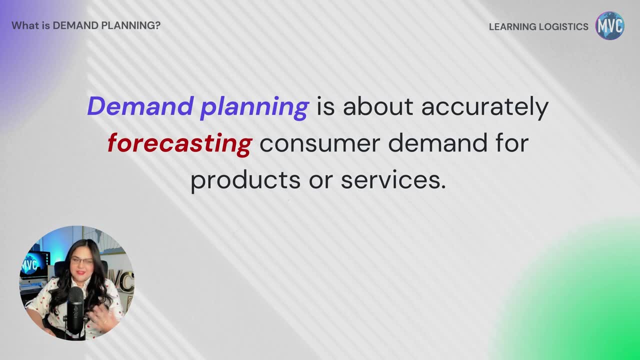 some effective demand planning and strategies And what those are strategies look like. right At its core, demand planning is about accurately forecasting consumer demand for products and services. Now this involves analyzing past sales data, analyzing market trends, and it also involves getting some 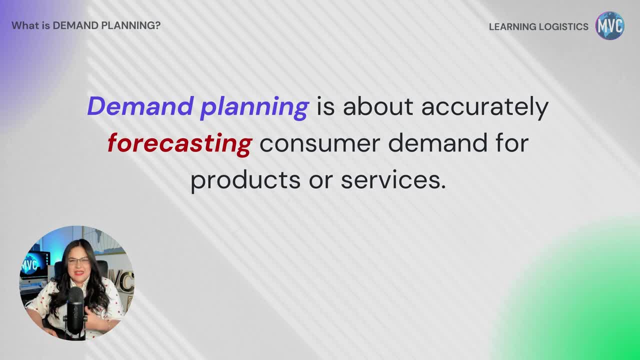 customer feedback to identify some patterns and so we can anticipate future demand. By forecasting demand, businesses, as I mentioned, can really ensure that they have the right inventory levels. you know that they can really meet the customer's needs without having issues of buying too much. 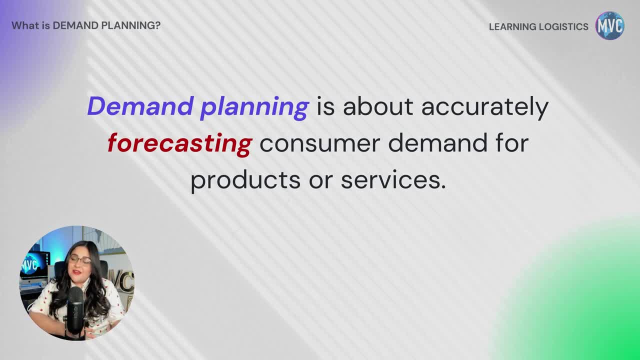 inventory or overstocking or not getting enough inventory or understocking or having stockouts- or at least that is the goal for companies within demand planning, and why it is so crucial for people within supply chain. We really want to know what is, or what can we expect the future demand for our products to be and how can we plan accordingly to that. 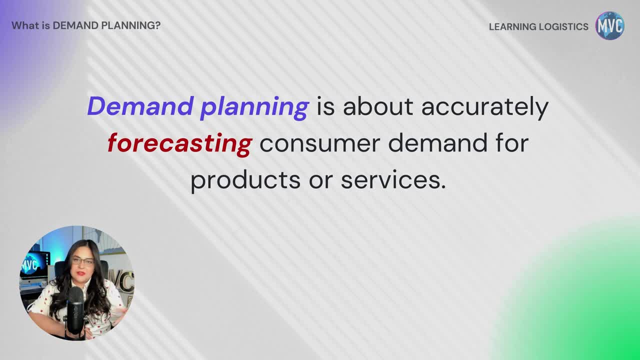 Because if we don't take this as one of the first or the earlier steps within supply chain, then we're really sort of going in the blind. We're not having a plan as far as how much we need to produce of something so that we can actually meet the demand and not lose money in the process. 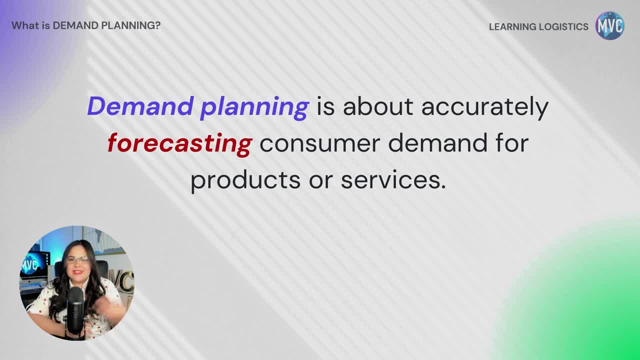 Think of yourself going back to your early days, of having to, you know, do a candy sale or a lemonade stand sale. You really needed to know how many lemons am I going to have to buy? How much candy am I going to have to get? 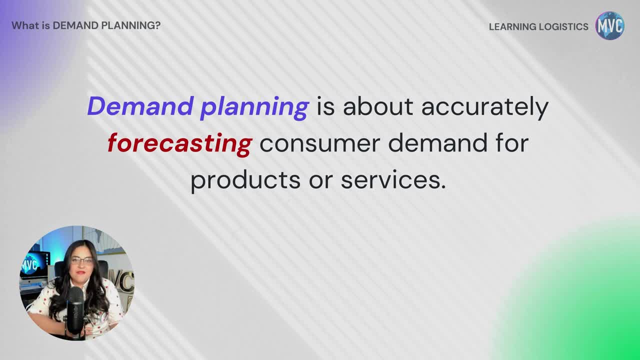 Is it going to be enough for the demand? Am I not going to have, or am I going to have too much? At the very early stages and when you're just starting out your business, it might be tricky to do that. Then you might not have those sort of factors, like I mentioned. past sales data. 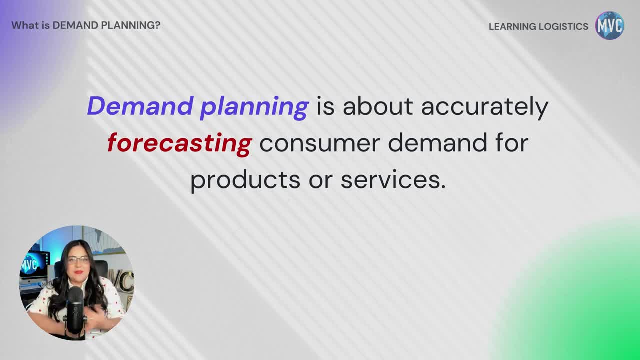 You might not have access to that because you're still just opening your business, or you're. you know you don't have a good idea of what you're doing in the business, yet You don't have any sales numbers. What you do in those sort of cases is use other types of data. 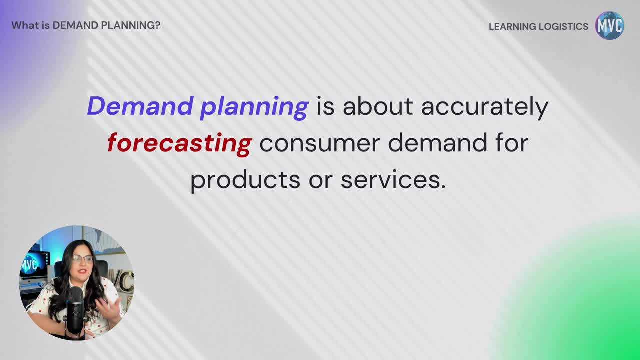 You use data within the industry that you're going to see. Well, if you wanted to sell lemonade- and this is your first time doing it- how about you ask your neighbors if any of the other people around the block had sold lemonade before and see what their numbers on their sales were? 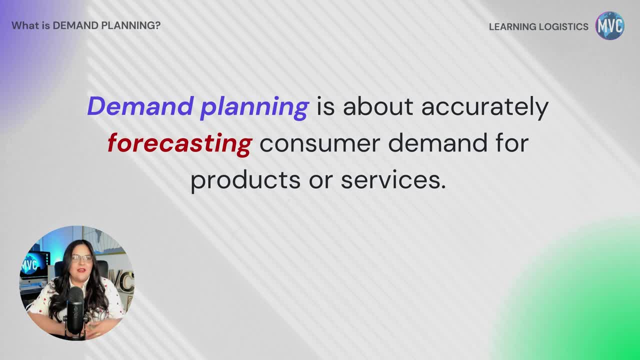 You can ask them what was the best time of the year to sell lemonade. You know, what did they usually have as far as clientele for the lemonade stand. So you can see how, in basic terms, we have to sort of figure out a way to know ahead of time how much of one item. 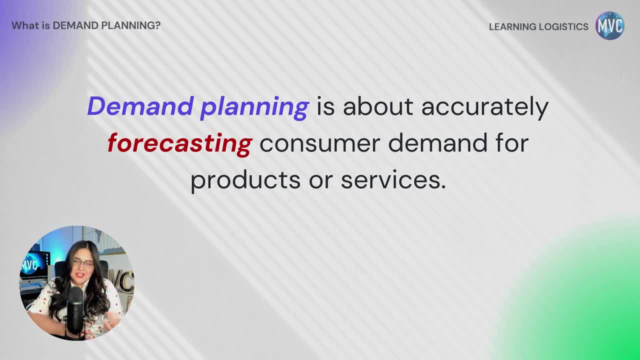 one product or how much of a service we're actually going to need before we actually set our plan in motion of selling something. So it makes a lot of sense once you look at it from that perspective, And it's just as I mentioned to you time and time again. 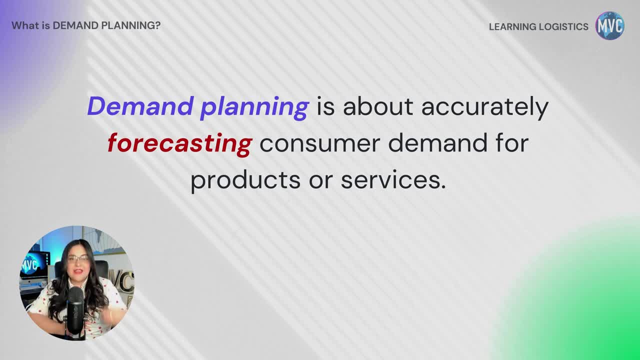 the supply chain is really about planning and having a plan ahead of time, or having a plan before we actually set anything else in motion. in the planning We want to forecast. what does it mean by forecast? I've mentioned this already in previous lessons. Forecast is sort of trying to predict. 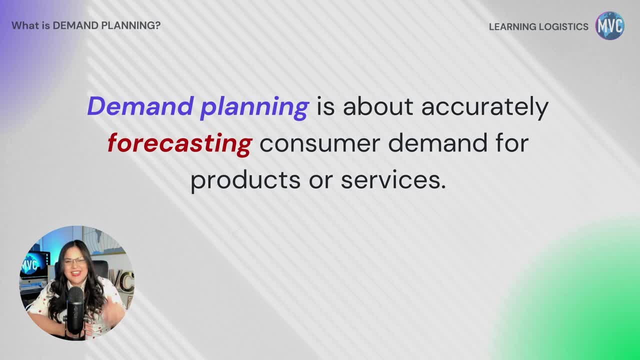 trying to foresee the future- we're fortune tellers here- or foresee the future In a way that we can do. we can implement that into our production schedules, into our manufacturing schedules, into our distribution processes, And I'm going to take you through those as we progress through the lesson today. but 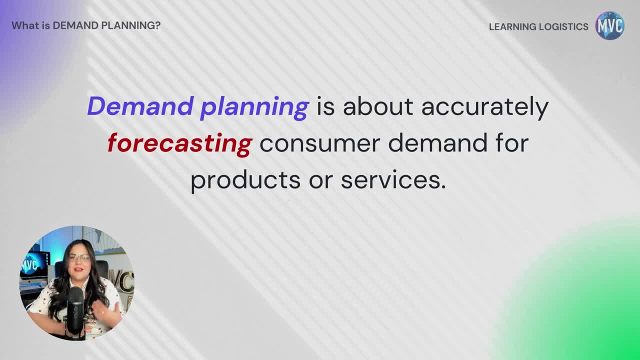 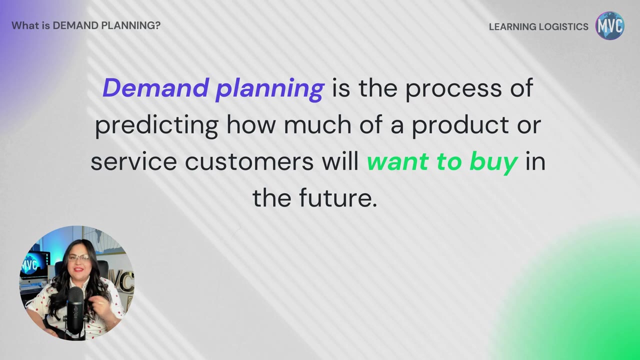 that would be the foundation of it. Demand planning really is about foreseeing, forecasting, predicting how much demand the consumer will have for our products. In simple terms, demand planning is the process of predicting how much of a product or service the customer will want in the future. 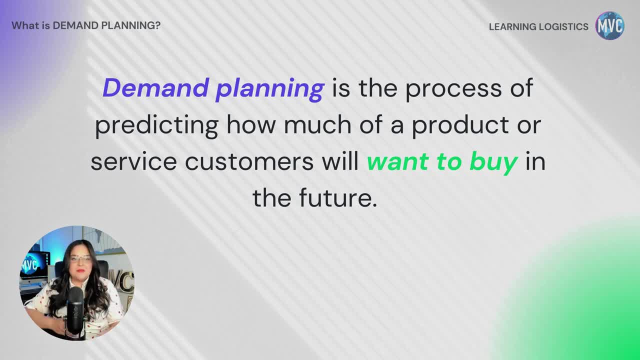 This will help a business prepare by making sure that they have enough inventory on hand to meet customer needs, without overstocking or buying too much inventory, or without understocking, which means not having enough inventory, which is also sometimes known as a stocking. 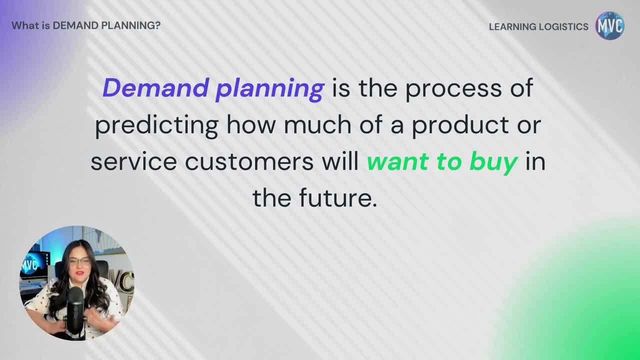 The demand planning involves using historical data, using market trends and other resources of information to make a forecast of future demand. We call this type of information, we call it quantitative data and qualitative data. Quantitative data is really the historical numbers, the sales data, the numbers in this. 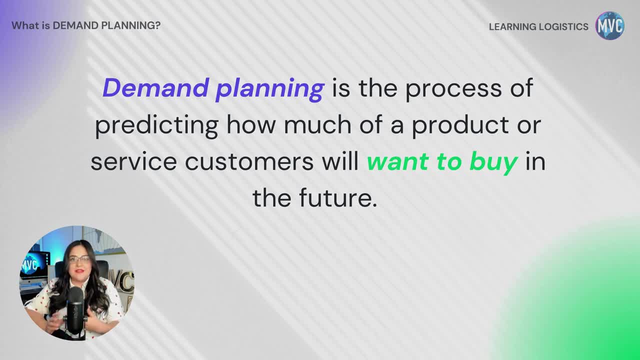 sort of equation for demand planning. The qualitative data is stuff that you would go out to an expert And have an expert's advice in the field or in the industry. try to help us figure out what the demand for the product will be in the future. 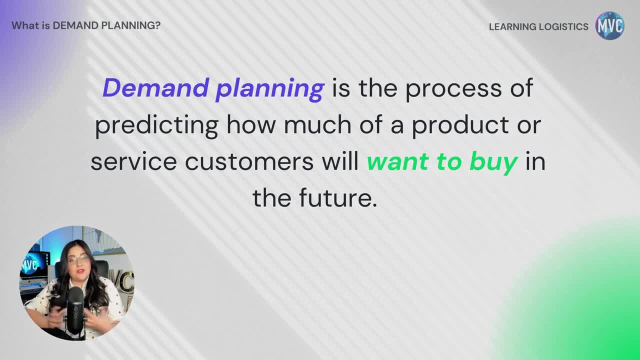 The companies that do it best. they sort of use a mix of the two. They use quantitative data as well as qualitative data, meaning we use the historical, the sales numbers, And we also look at what the experts are saying. what are some of the trends that we see out? 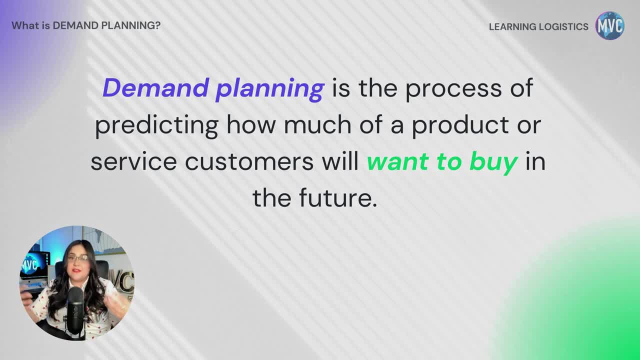 there. Where do we see, like the experts in the industry telling us that the market is going to next? That's what we mean. So we combine sort of the two and then we make the best educated guess for our companies as far as what the demand for the product will be within a particular time frame. 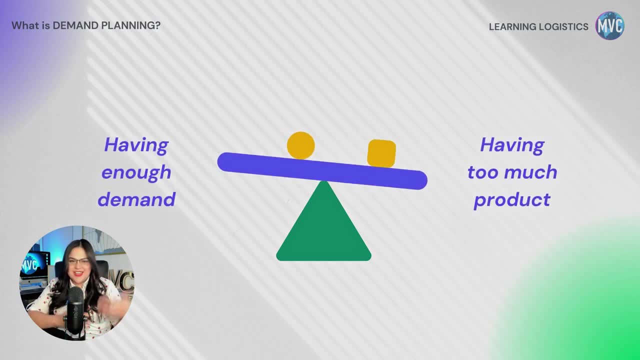 Now, as you can see, sort of in this teeter-totter, see-saw kind of situation, we really want to do is balance two things within demand planning. The goal here will be to ensure that the business is prepared to meet the customer's needs. 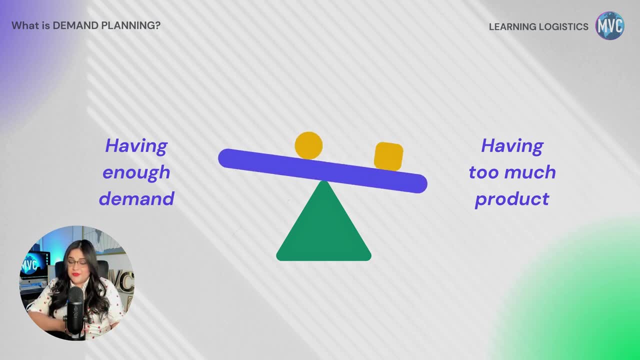 but also avoiding situations where you run out of stock or you have too much stock to sell. It is really a balancing act between having enough demand in one end and also having too much product on the other end, And demand planning and people that work in this area or in this particular department. 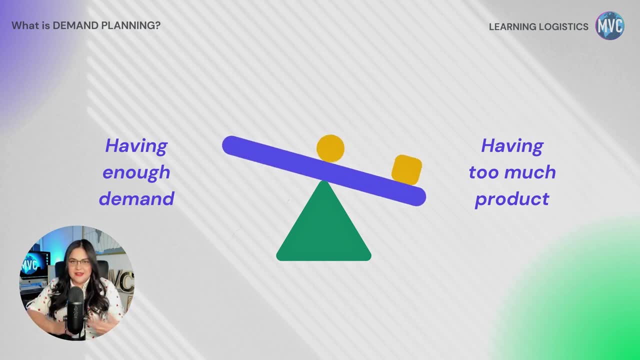 or section of supply chain will tell you really is a balancing act. You never want to run out of product where the customer is placing an order and you don't have enough to, And then, on the opposite end, you don't want to buy too much of a particular material good. 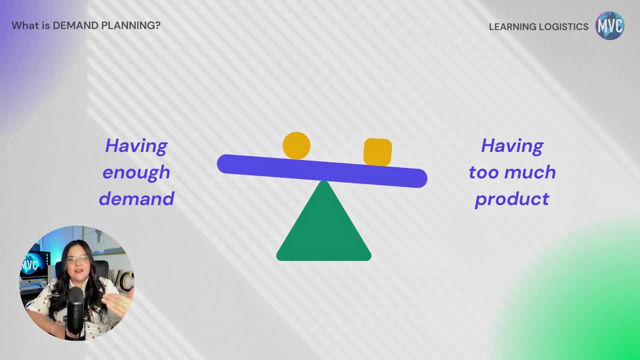 or make too much, that the product is spoiled, the product could be damaged or the product could run its lifetime and that you might not be able to sell it for a profit, And that's also the difficulty in it. So, yeah, we have this sort of balancing act in demand planning and people that work there. 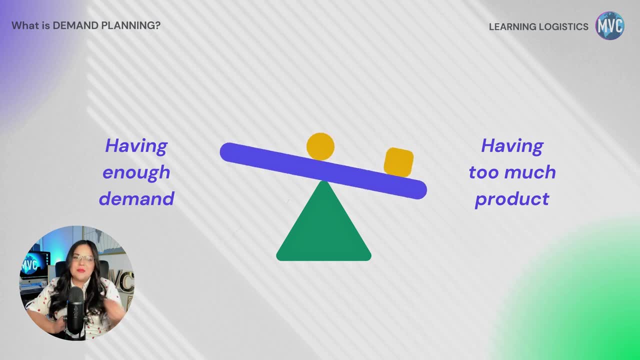 will tell you that it's everything. It's about the very subtle balance between getting too much inventory, where you're not going to sell all of it, or not having enough inventory, where a customer comes in and places an order Okay, And there's so many factors. we just saw within pandemic when stuff hit and closures were. 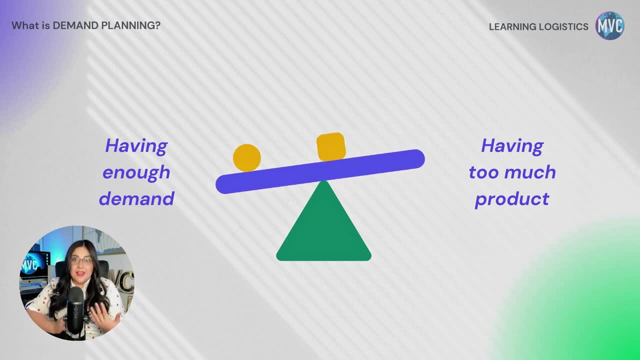 coming down and lockdowns weren't happening. That sort of balance in demand planning really really shifted. There was not enough demand for certain goods and items because we were going to sell a lot of goods and items and we weren't going into lockdowns and people were staying at home. 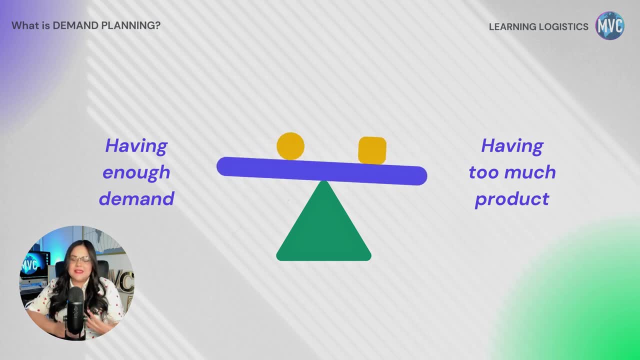 They weren't having to go out into the road anymore, They weren't able to travel, go places. you know, we all saw that. And then, on the opposite end of things, we had an increase in demand for other goods and items, you know, sanitary products, PPE, stuff, that was necessities- were really increased. 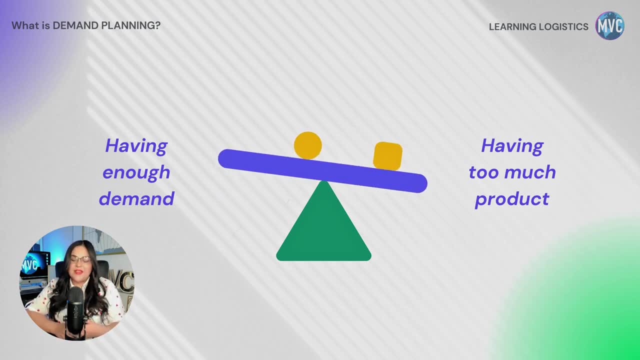 in demand because we all needed those products right away. So then there was the issue with the supply. We weren't having enough of them Because previously, or prior to the pandemic hitting or starting, we had a different level of demand for those goods. 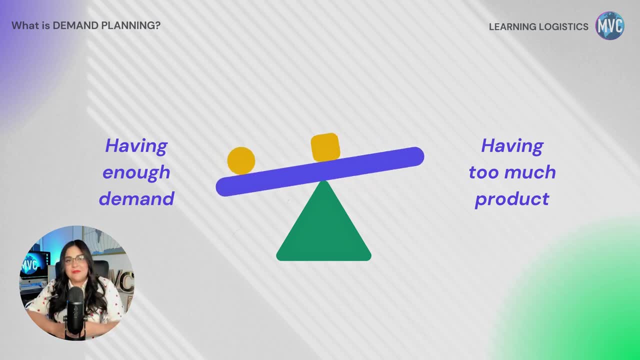 So supply was at that particular level to meet that demand. When demand really spiked for those products there wasn't enough out there to supply those goods. Companies weren't manufacturing to those goods, to that idea or that level of demand. when we hit the pandemic and we hit the lockdowns, 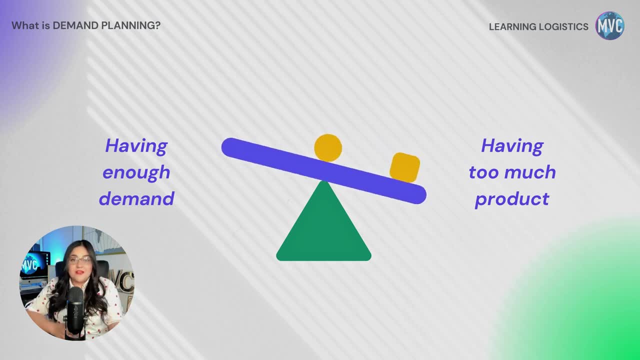 So we all were witnesses on that. right, You went to the store And there wasn't enough toilet paper. That was because companies were working off a certain demand level and they were planning their production and their distribution of the toilet paper products at a certain level. 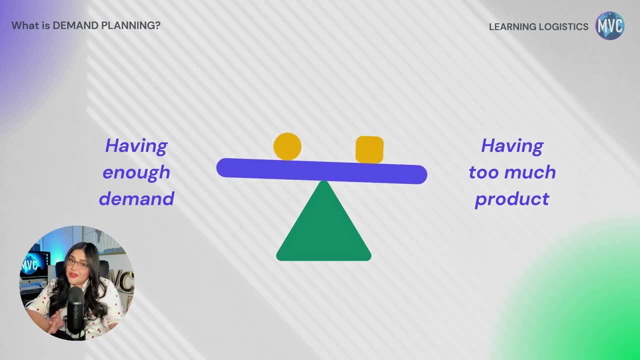 When pandemic hit and we all went into a frenzy of not having enough toilet paper. believe me, I did go through that myself, But we went through this sort of panic of buying so much toilet paper that we were unable to make enough as fast as the demand was being provided. 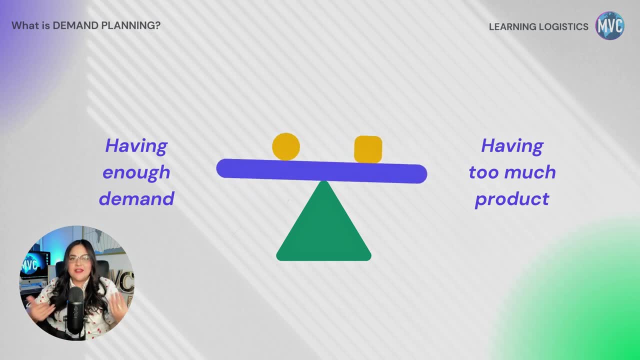 And now we see demand levels that are more evening out. We have also inflation and other economic factors that are affecting the market out there. But as a business, what you have to do is be very, very aware of these issues affecting your market and be able to sort of adjust to that as you progress in your demand planning. 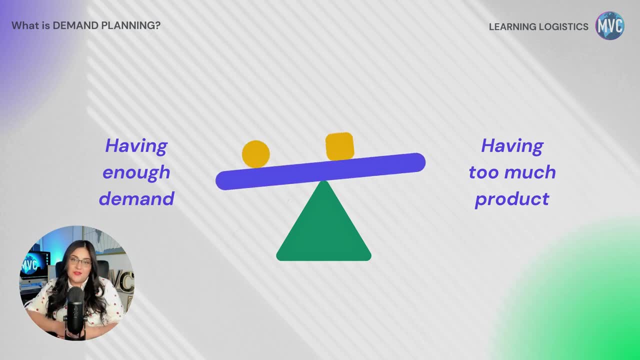 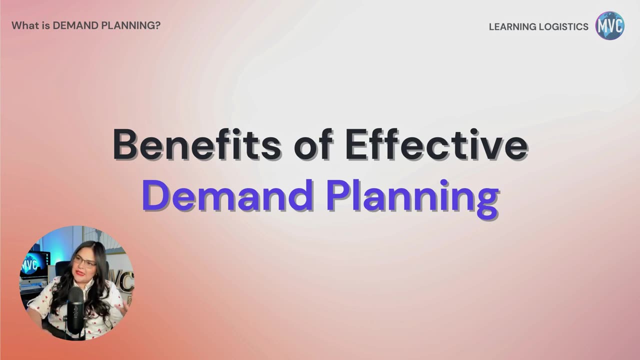 schedules and also as we move into the production of those goods. So in this section we're going to talk about the benefits. Okay, How effective demand planning. Now we know what it is, what it's good for, but we also need to understand that we need 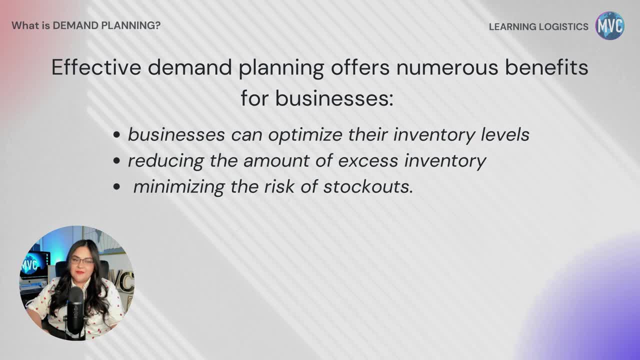 to do it well. So when we do it effectively, it really can offer a numerous amount of benefits for businesses. We can, by accurately forecasting demand, businesses can optimize their inventory levels, They can reduce the amount of excess inventory and they can minimize the risks of stockouts. 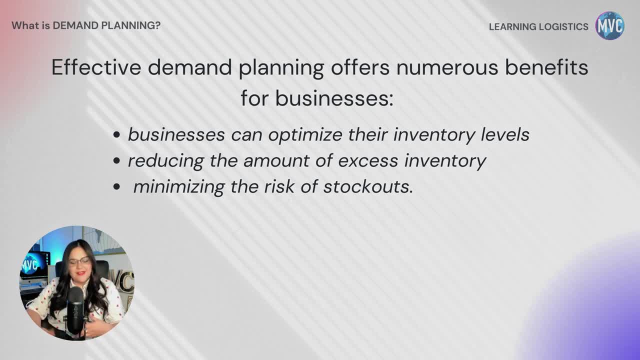 This, all summed up, can really lead to cost savings and it can improve customer satisfaction. If we're not tying up as much money in inventory because we know exactly what to buy and how much to buy, then we're having a better cashflow in our business. 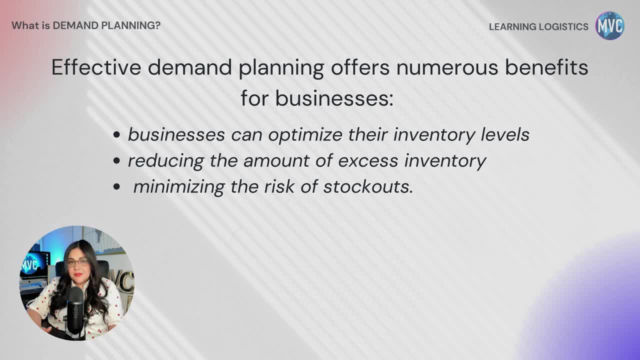 If we're having products as customers place orders. the customers are going to be happy with us. They're going to know that they can rely on us. They can depend on us. They can trust us to have the levels of inventory we need to be able to fulfill the demand. 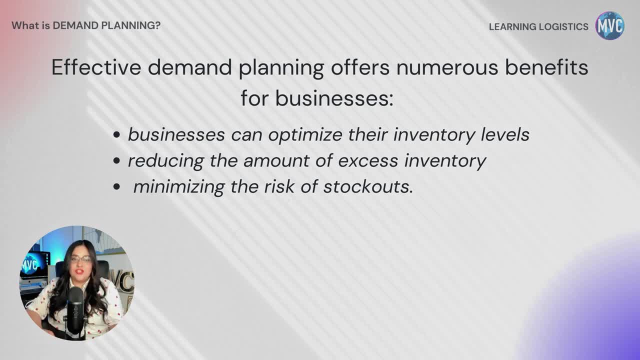 Okay, Okay. So we need to be able to fulfill our needs and have a little bit of a cushion in that sense, And that always keeps customers happy, right? Because we need to be able to fulfill their needs very quickly and efficiently, because there's such a competitive market out there for basically all products that are in the 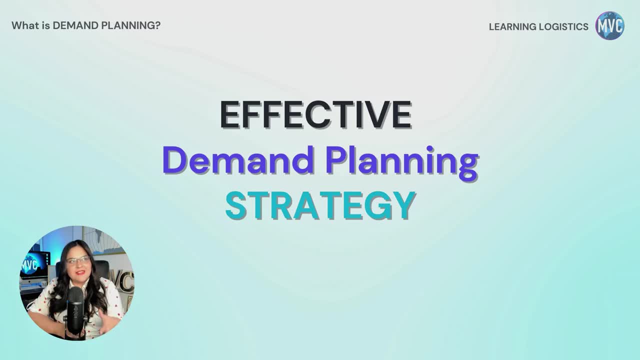 market, Okay. So you're telling yourself: okay, professor, I think it sounds all nice and great and fancy, but how do we actually do that as a business? or how do I, as a student, learn to do this? Well, that's what we're going to talk about. 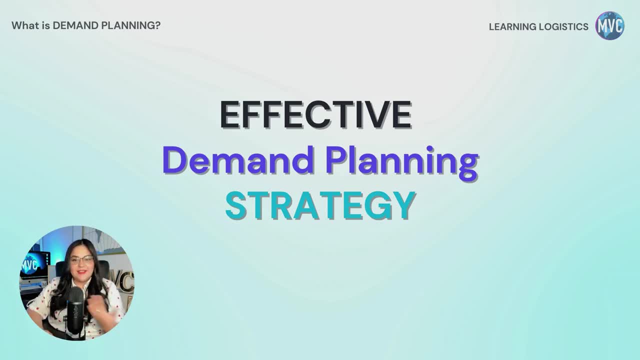 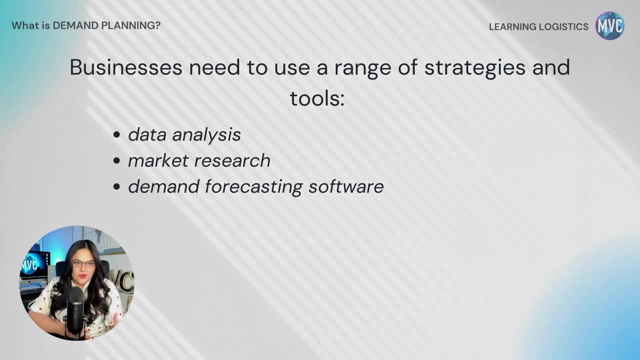 In this section, we're going to talk about effective demand planning strategy. To implement effective demand planning strategies for your business or for the company you work for, we're going to really need to know about certain strategies and implement certain tools. These may include data analysis, market research and using demand forecasting software. 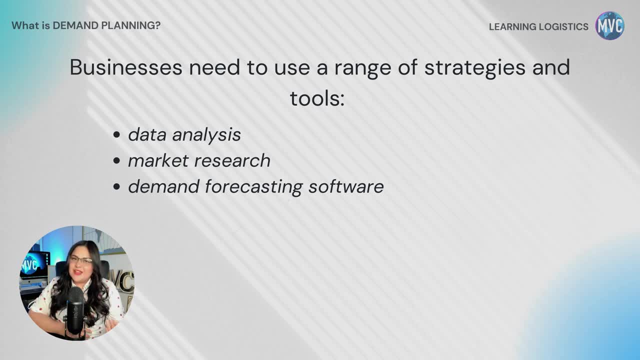 It's also important to have a flexible supply chain that can really control the demand. So we're going to talk about effective demand planning strategy, Okay, Okay. So we're going to have a flexible supply chain that can really quickly adjust to changes in demand. 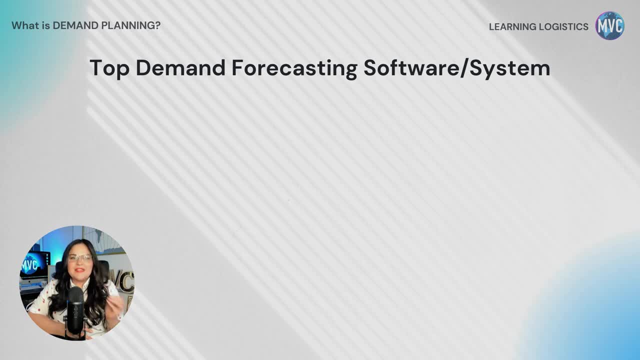 Now here I'm going to tell you what are some of the top demand forecasting software providers that are out there, and some of the ones that I'm familiar with, that I've used in the past, some of the ones that some colleagues have used as well, and also for some of the research. 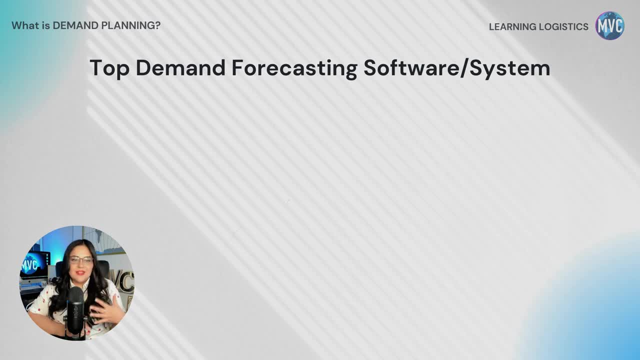 that I've done on my own, on my end, So I'm going to give you a list of them, right, Okay, So this is nothing biased, I'm just not going to rank them, I'm just going to give you a. 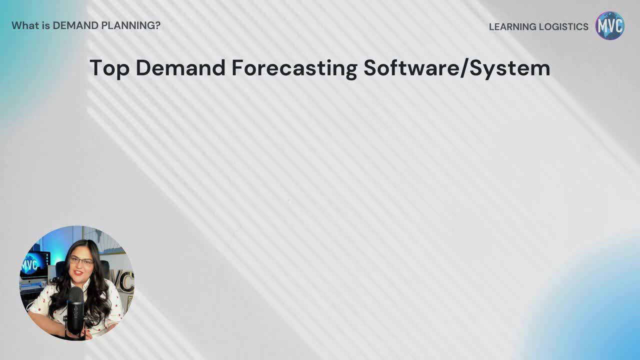 list of what are some of the demand forecasting software providers so that you can learn more about them, And I'm going to tell you where you can find some free, or relatively free, courses on those softwares. Okay, So here we go. So the first one that we have is SAS Forecast or SAS Forecast Server. 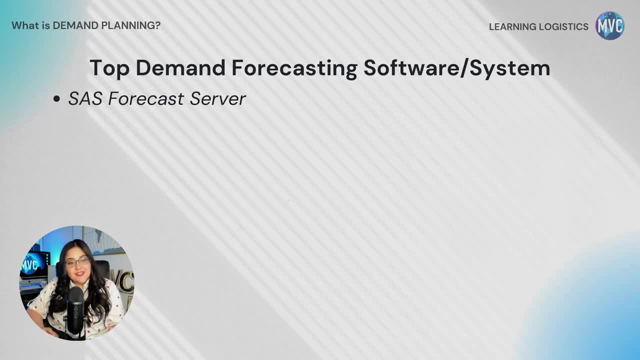 Now, SAS offers a variety of free courses. Okay, So the first one that I'm going to tell you about is the SAS Forecast Server, which is a software that you can use to do on-demand forecasting, including courses on forecasting methods, time series analysis and data preparation for forecasting. 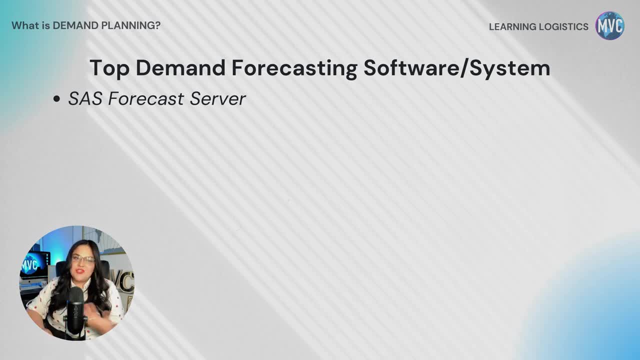 These courses are available through their own website. So you do, if you want to implement this software for your company, your business, you do have to pay for these services. You have to pay for these software or these systems, But if you want to learn about them, because, say, your company that you work for, or the 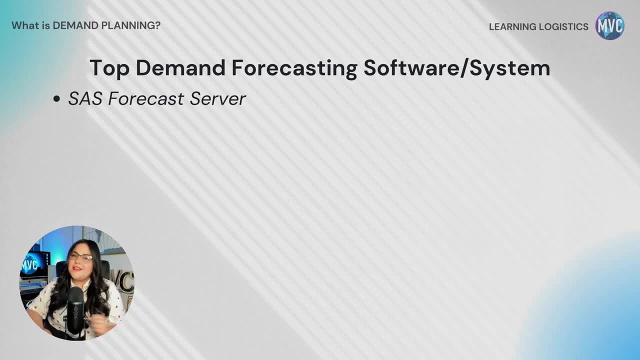 business that you work for. they want to use it. Okay, They want to use this or something similar. You can always get access to courses on how to do that and become more familiar with it. We also have the trusted and very old school Microsoft Excel. 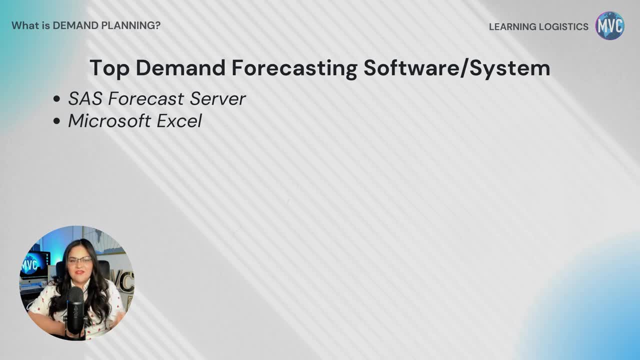 Now, while Excel is not dedicated exclusively to demand forecasting, it can be used to perform basic forecasting tasks. Now, Microsoft offers a range of free courses on Excel, including courses on forecasting and time series analysis, So you can always Google those or check those out. 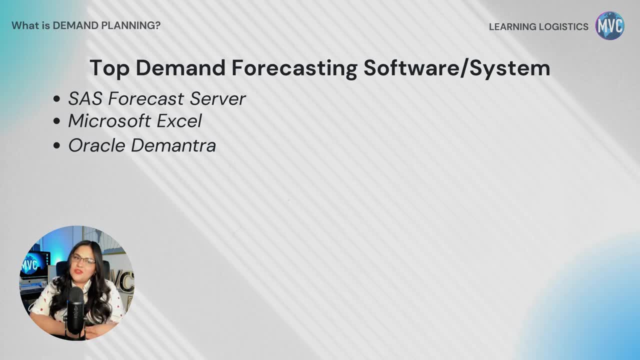 The next one that I'm going to talk about is Oracle Demantra. Now Oracle offers a free trial of the Demantra software, which includes a range of demand forecasting tools. So this is something that your company has been looking to get into, or get into their 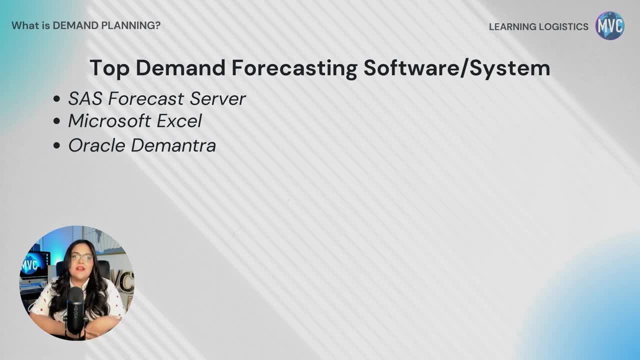 operations and implement a demand casting software, while Oracle offers a free version or a free trial- Okay, I shouldn't say version, I should say trial, a free trial- of their Oracle Demantra system. They also have a variety of courses on demand forecasting and supply chain planning through 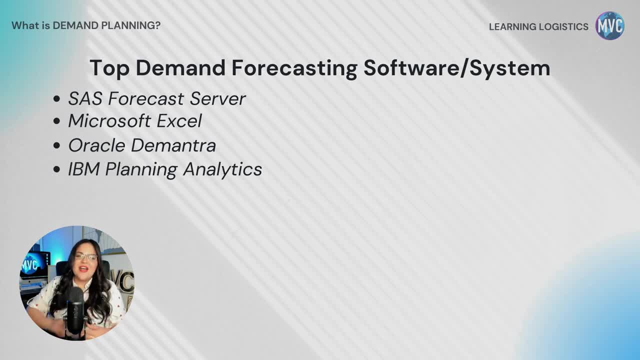 their Oracle University. Next, we have IBM planning analytics. IBM offers a variety of free courses on this platform on demand forecasting and planning through their IBM skills gateway. Now these courses cover topics such as time series, forecasting, predict analytics and demand planning. Next, the next software is SAP or SAP. I call them SAP. I hear people say SAP. I hear people. 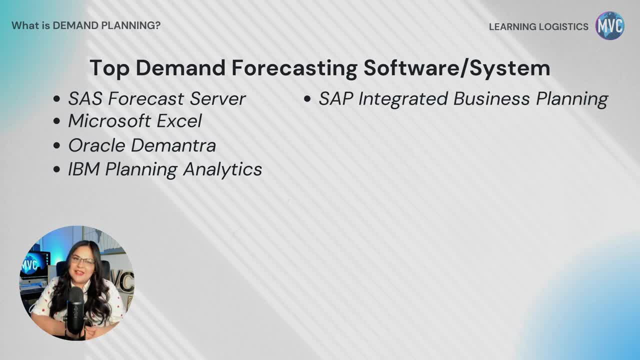 call SAP. We say SAP, SAP- integrated business planning. now SAP offers also- and this is a type of demand forecasting software that they offer, but they also have courses for you to learn about the demand forecasting and planning features within this system. Now you could learn this about these courses through what is called the SAP learning hub. 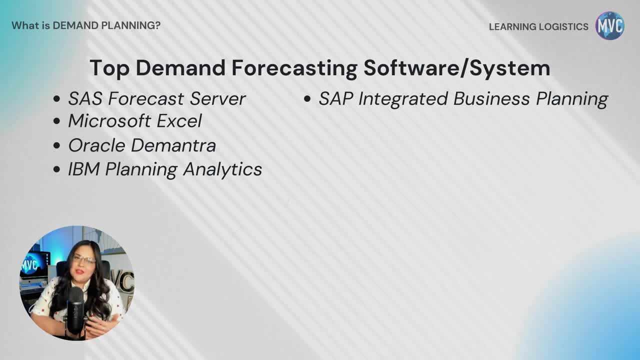 While some courses do require you to have a paid subscription, they also have other free courses on demand forecasting and sales and operations planning. Up next, we have Tableau Now. Tableau is a data visualization software that can be used for demand forecasting and 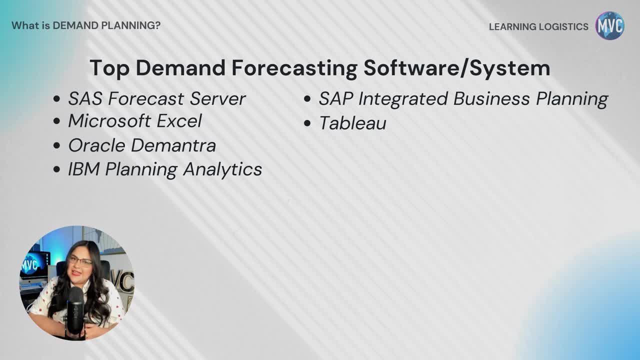 they do offer a variety. They offer a variety of free courses on data analysis and visualization which can be useful for forecasting people and they can be useful for people working in this sort of industry. All right, so this is very data driven tasks and you're able to figure out more visually. 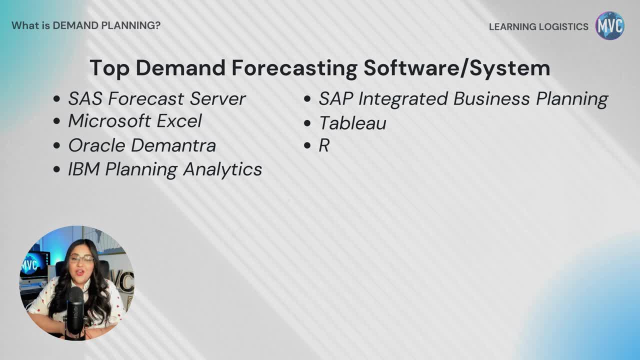 what your demand planning might look like. Up next we have R. R is free open source software for statistical computing and graphics. It includes a range of libraries and packages for demand forecasting and for also for time series analysis. Now there are many free courses and resources available for learning R, which includes the 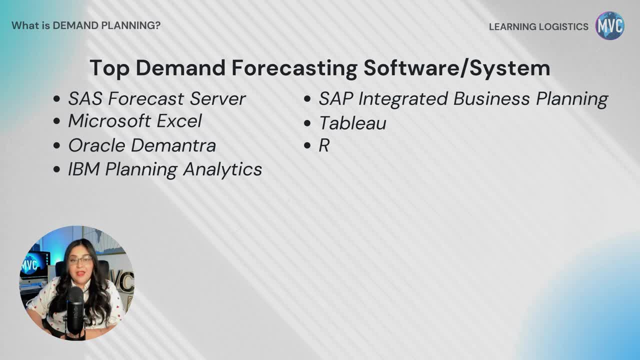 R project website and various online learning platforms, like in DataCamp and also on Coursera. Finally, we have Python. Now Python is another very popular language for data analysis that can be used for data analysis. It's a very popular language for data analysis. 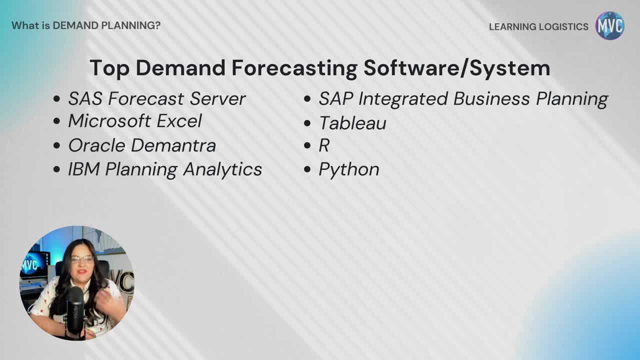 It's a very popular language for data analysis. It's a very popular language for data analysis. It can be used for forecasting as well. There are many free resources available online for learning Python. I've started and I'm still in that process, and I could tell you that it's easy enough. 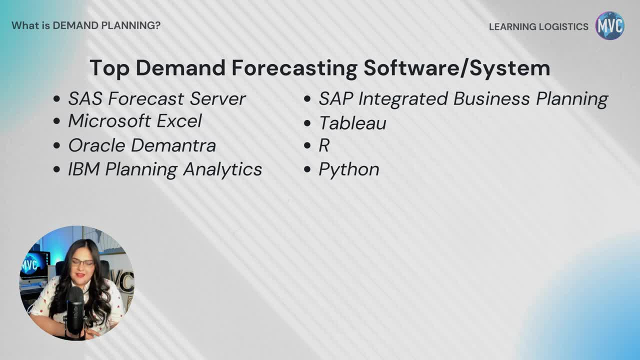 once you get the hang of it. Now, these can include courses like Coursera courses, EVX courses as well. Some of them are free, but you do have to pay to actually get the certification once you finish the course. But if you get the course for free, you're learning about it. 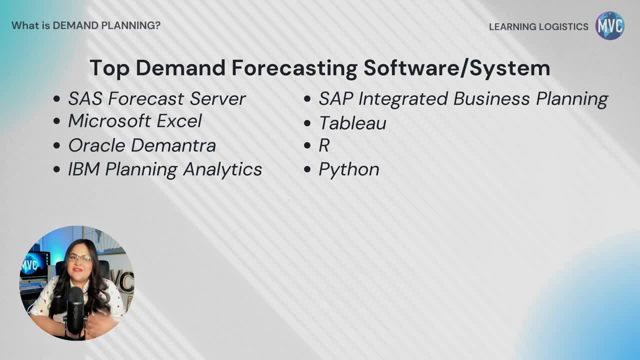 So why not? And Code Academy, as well as various tutorials, tutorials and guides that you can find online here on YouTube, which are all very great, So you can check those out as well. I will say, and it's very important for me to note that the man 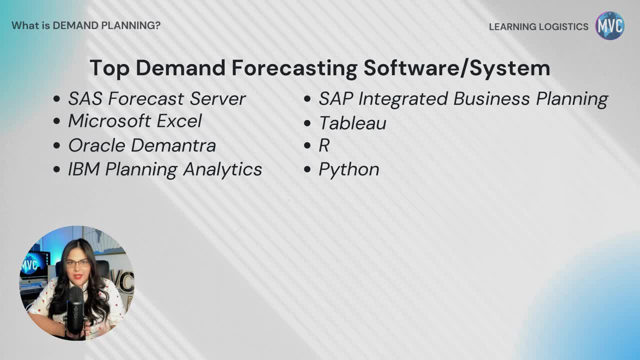 planning. software and systems can really vary widely depending on what industry you're working in the terms of the costs, how complex they are and what are the features of these systems. Now, the software systems that I've listed below may or may not be suitable for all businesses. 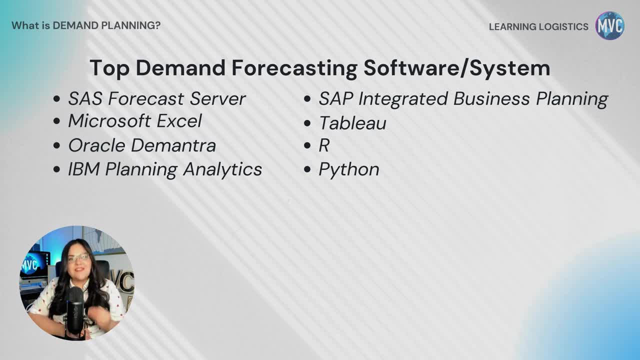 So it is important to do your own research and to evaluate each of them and give them you know your own grading, your own review, based on what the needs are for your specific business, what are your goals, what are your needs- and based on what you're going to implement this. 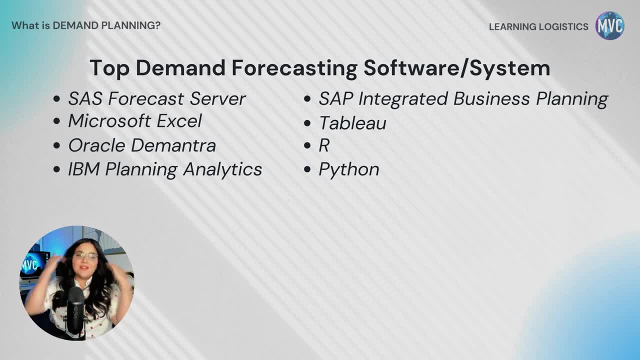 software for All right. this is just like a broad review of them, So you could get a better idea of what is out there if you weren't too familiar with All right. so this is as far as technical as I get. We will continue to move on in the lesson with what's next. 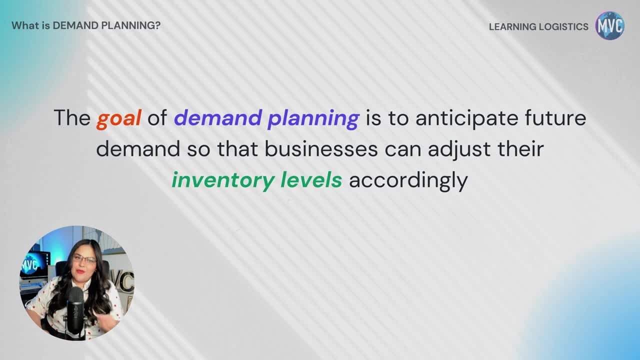 The man planning is a complex process that involves predicting consumer demand for products and services. We have established that Now the goal of the man planning is to anticipate future demand, so the businesses can adjust their inventory levels accordingly and also ensure that they have the right amount of inventory on hand. So that's the first step. The second step is to 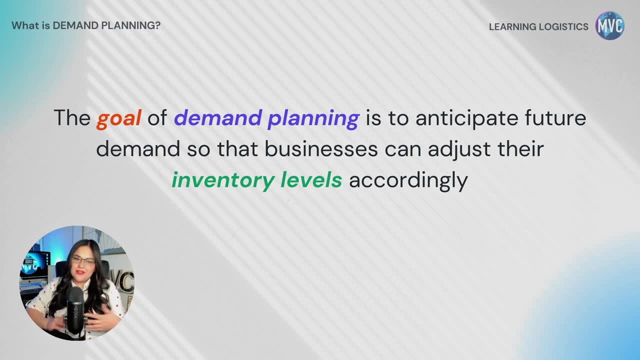 make sure that the business has the right amount of inventory on hand. And the third step is to make sure that the business has the right amount of inventory on hand. And the fourth step is to to meet customer needs without having too much or not enough, which I mentioned earlier in the 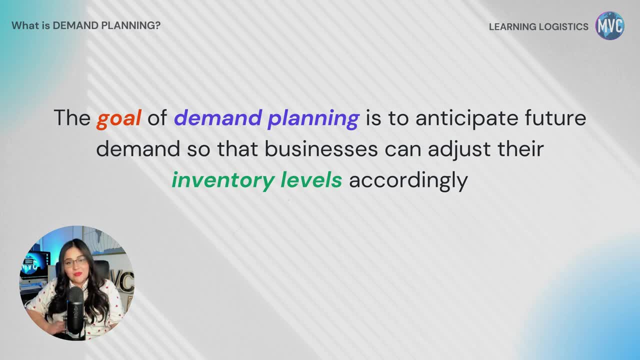 lesson. So, ultimately, just keep in mind that the goal of the man planning is really to anticipate future demand. Some of the software systems that I mentioned earlier helps us do that by inputting data, sales numbers, anything that we can find as far as quantitative data So we can take out of. 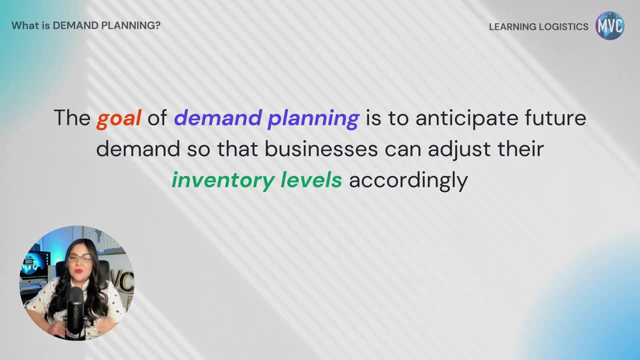 that equation And then we can take out of that equation and we can take out of that equation and the result as to what we might think the levels of inventory might be in the future, based on previous data, sales and historical information. In this section we're going to talk about the key principles of effective demand planning. 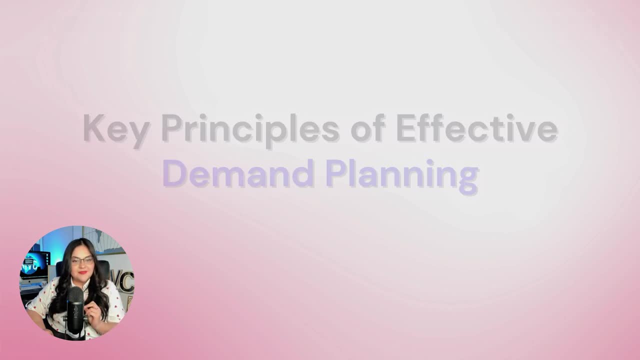 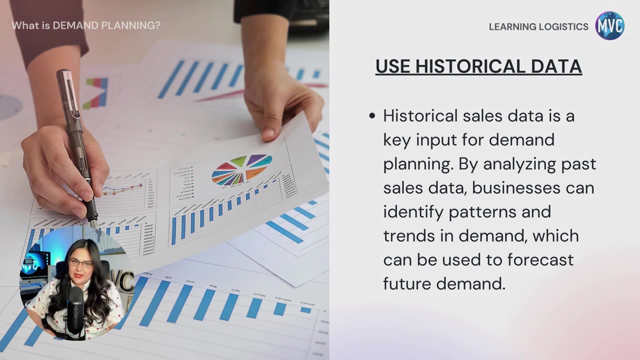 Of effective demand planning. a first is to use historical data. Historical sales data is a key input for demand planning. By analyzing past sales information or data data, sales and historical information that the business will be behind data, businesses can identify patterns and trends in demand which can be used to forecast. 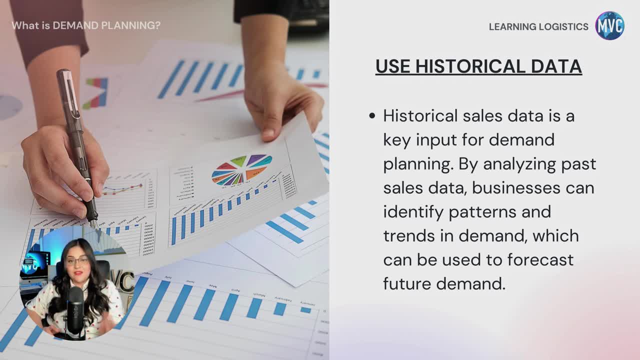 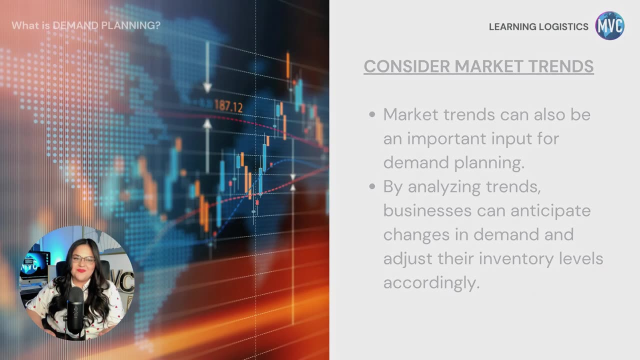 the future demand. It is important to ensure that the historical data that is being used is relevant, also accurate, as this can greatly impact the accuracy of the results, meaning the actual demand forecast. right Next is considering the market trends. Market trends can also be a very important input for analyzing demand and for planning. 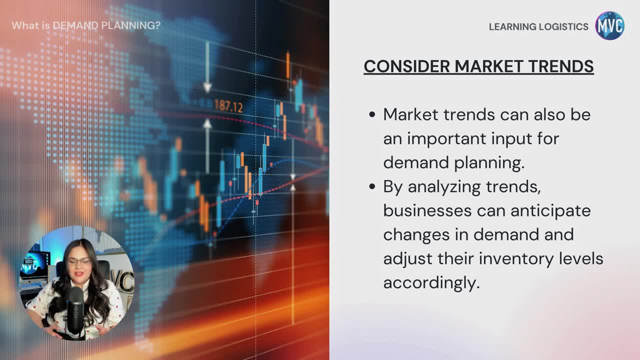 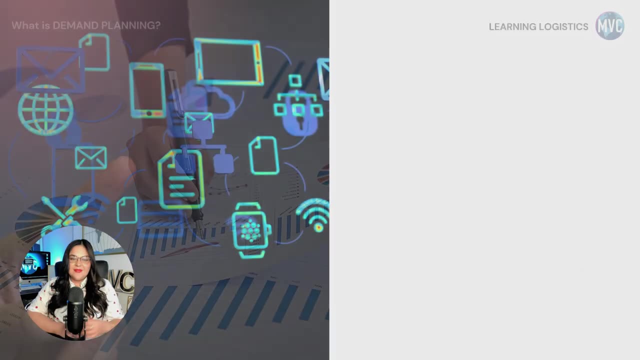 our demand. By sort of taking a look at the trends in the market, such as changes in consumer behavior or the emergence of new competitors, businesses can really anticipate changes in demand and adjust their inventory levels accordingly. Another key principle is to use multiple data sources. 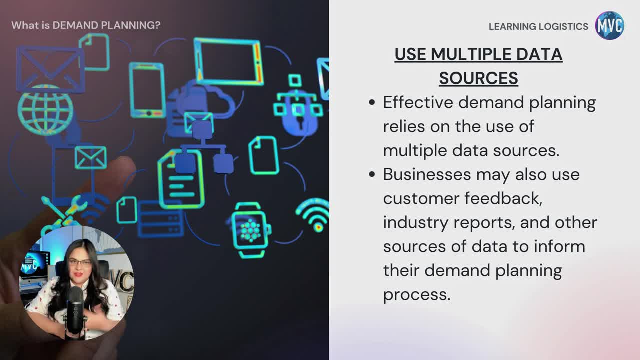 Effective demand planning Relative. In addition to historical sales data, which we established is very important, and to the market trends, business can also use other things, such as customer feedback, industry reports and other sources of data to inform their demand planning process or to input. 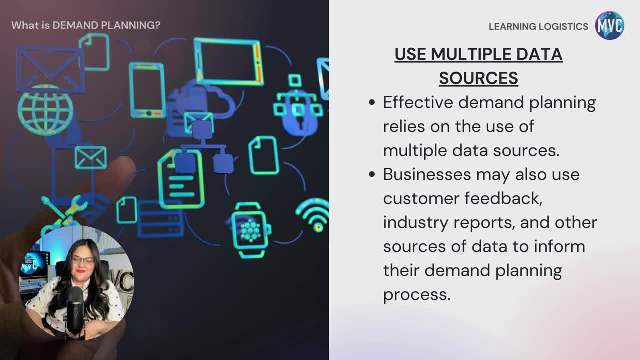 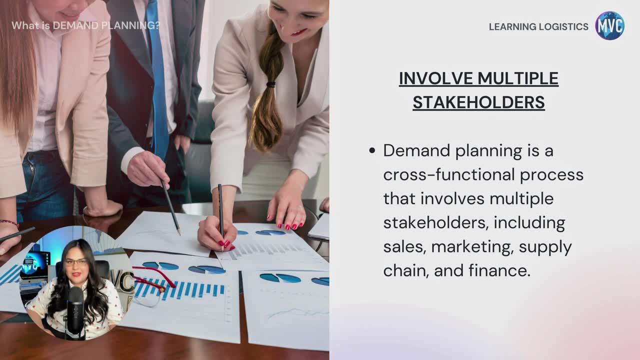 into their systems. Next is involved multiple stakeholders. Demand planning is cross-functional Process that involves multiple stakeholders, including sales, marketing, supply chain management and finance. It is important to involve all these relevant stakeholders or departments or areas and the demand planning process to ensure that all the perspectives are being considered and that the 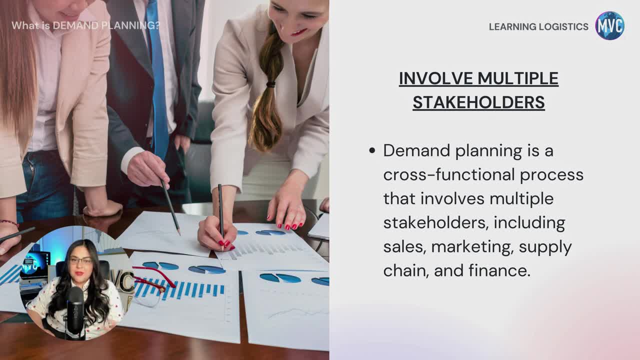 demand forecast is accurate. Another thing you learn about supply chain in some of the next lessons is that the demand plan, The demand plan sort of swifts his way or pushes his way into the supply plan. meaning once we figure out how much demand we'll have, that will end up in how much we plan to produce. 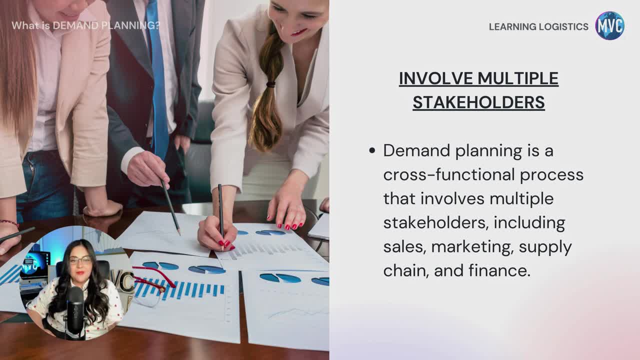 and that's called a supply plan. So without a demand planning place that everybody can agree upon, everybody can be in a consensus about within all these different departments that include all these different stakeholders, If we can't come to a consensus on one single demand plan, you can't have multiple, you can only have one. 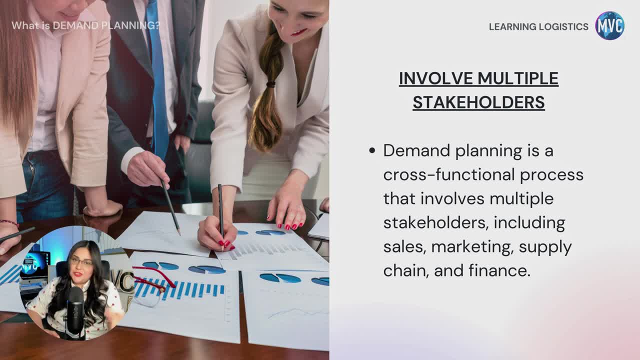 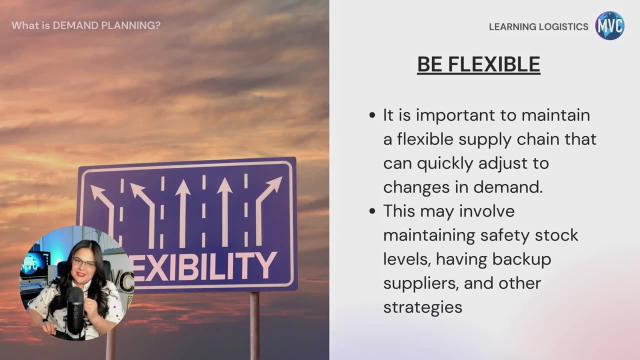 One single demand plan that is going to push forward into our supply plan that we can proceed, And that's something that is basic and what we know as supply chain management. So keep that in mind. Finally, be flexible. It is important to maintain a flexible supply chain that can quickly adjust to changes in demand. 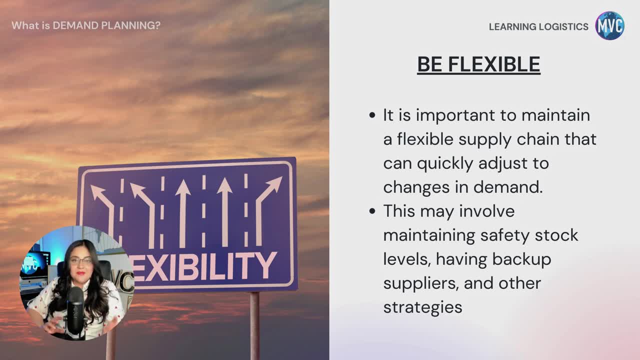 This may involve maintaining safety stock levels, having backup suppliers and other strategies to ensure that the business can respond quickly to changes in demand. If you watched our episode number seven, you learned about demand and supply chain uncertainty and some of the factors that cause disruptions in our supply chains. 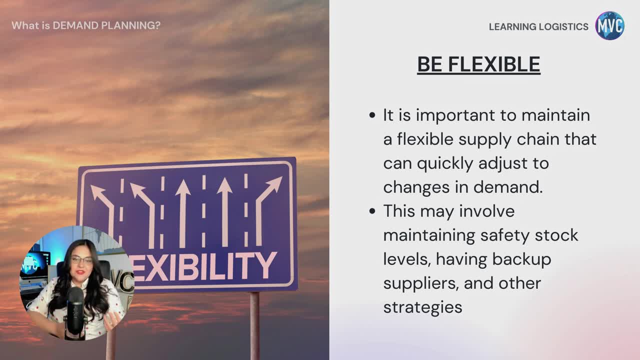 This also sort of carries along here, because when we're trying to plan for our demand, we need to know how to adjust to certain things that will disrupt our supply chains, And the purpose of being flexible or agile or responding quickly to changes is that so we can resolve those issues, those uncertainties in our supply chains. 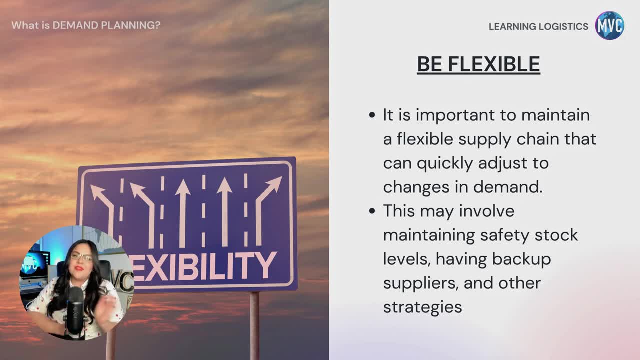 and be able to adapt to those changes. We also see that here in demand planning. So it's another principle. another key thing within demand planning is to be flexible, Because, yes, we do want to have a demand forecast and implement a demand plan. 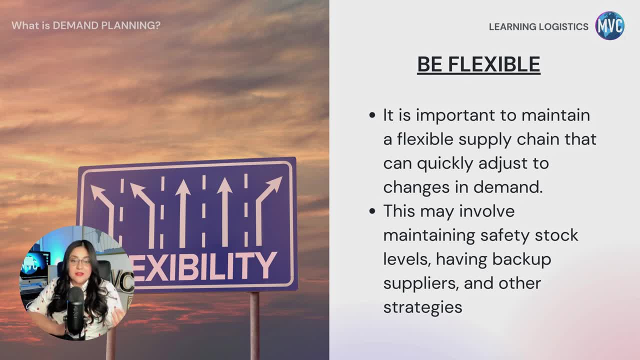 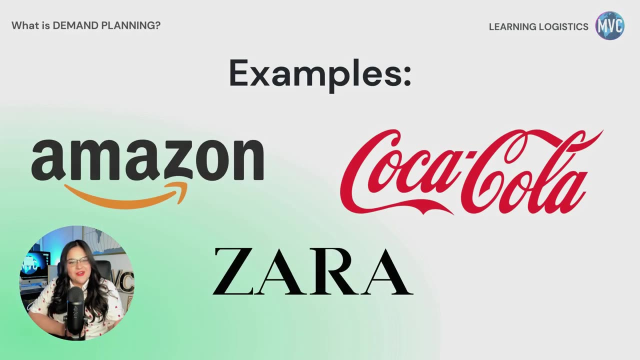 But if we see something that's happening and something that can majorly impact our operations or demand, then we need to be able to implement that and have ways to implement that as well. And now we've come to my favorite part of the lesson, which are the examples. 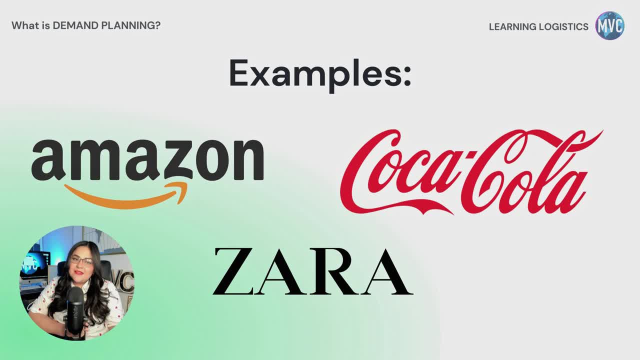 Now we're going to talk today about companies using demand planning. Many companies have successfully implemented demand planning strategies to improve their supply chain. I'm going to give you three examples of companies that have done that and how they have effectively used demand planning. So we have. today we're going to talk about Amazon, Zara and Coca-Cola. 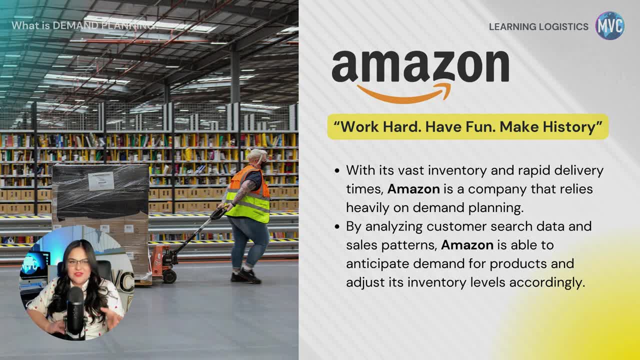 Okay, so first up is Amazon. Now, with this very vast inventory and rapid delivery times, Amazon is a company that relies heavily on demand planning. By analyzing customer search data, sales patterns, the company is able to anticipate the demand for products and adjust its inventory levels accordingly. 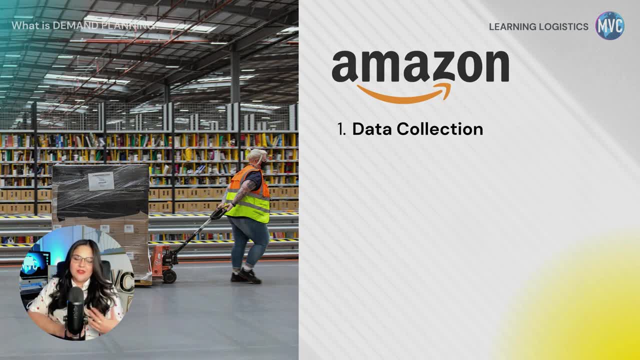 Okay, so here we're going to take you sort of by the step-by-step or the progression of how Amazon does this. because Amazon really does implement demand planning processes And they're a very crucial part of their operations. because, like I said, 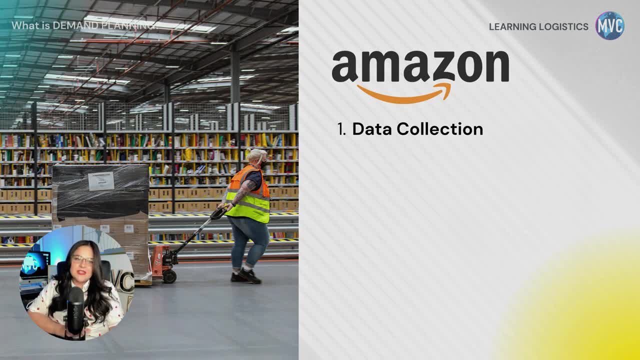 it helps you make sure that they have the right products for the right quantities and at the right time to meet their customer demand. The process involves a number of steps that are designed to help Amazon: forecast demand accurately, plan their inventory levels, optimize their supply chains. 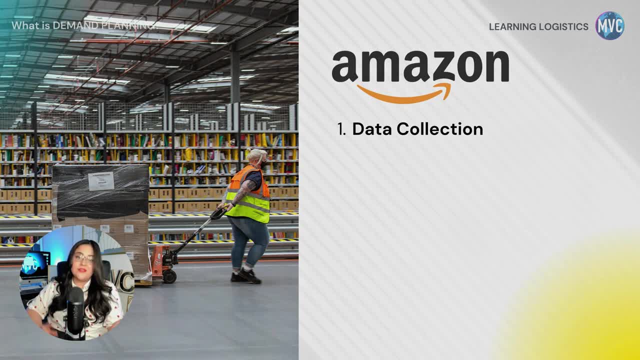 and to ensure that the products are delivered to the customers when the customers need them. I mean Amazon customers. we can say- and if you're familiar with Amazon, I'm sure you are- you expect fast delivery or you're expecting the product to get to you, based on how you order it. 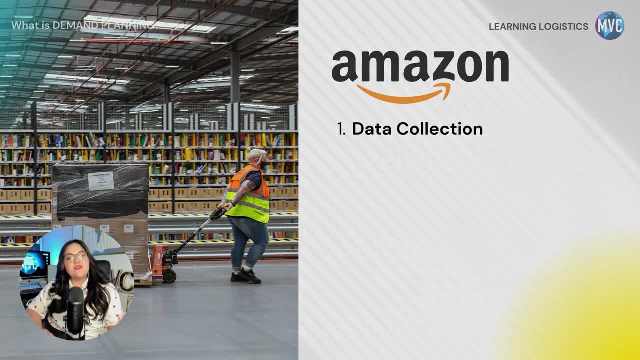 a day or two days, three days maybe. You're expecting sort of a faster delivery time on that. So here I'm going to take you through the step-by-step of how Amazon demand planning process looks like. The first thing is data collection. 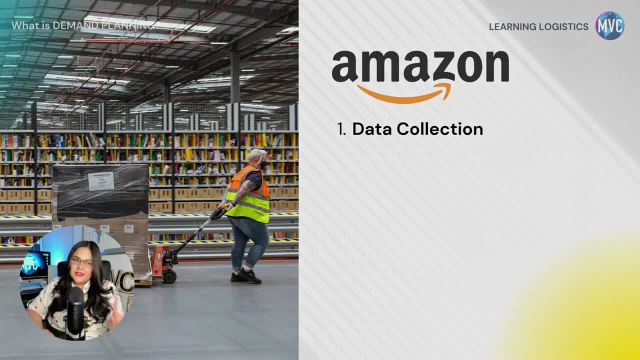 This is the first step in Amazon's demand planning process. They collect data from various sources. This includes sales data, customer feedback, market trends and other relevant information that can help them in their forecasting for the demand. Amazon uses advanced analytics and machine learning algorithms to process this huge amount of data. 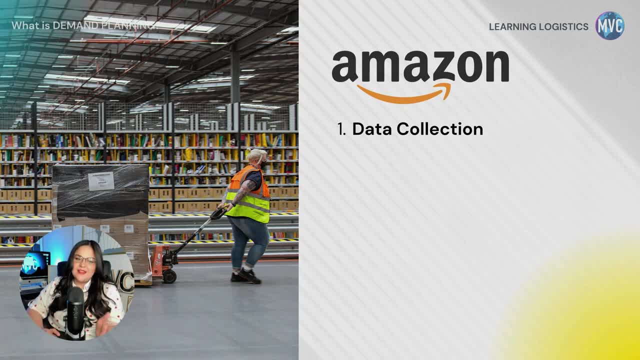 and to help them identify patterns and trends that can help in predicting future demand. If you've ever been on the website right or on the app and you've made a purchase and at the bottom of the section of the item that you're looking at, 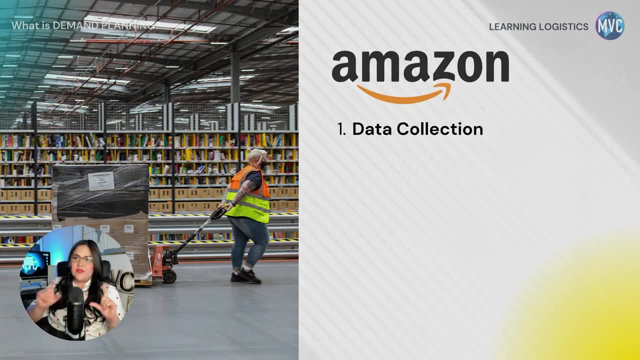 it'll tell you related items to the search or other customers have also purchased and it gives you a list of that right, Or it gives you a list of saying, based on your previous purchases, you might be interested in this and you can check those out. 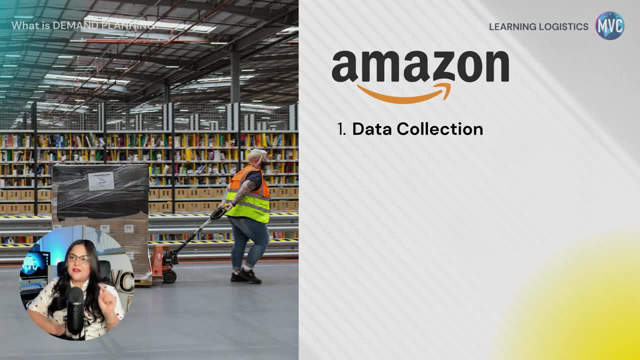 This is done based on your historical sales data, what other people in your area have purchased, what other people searching for the products that you're searching have also purchased, and any kind of information you have either on your profiles and your settings and on your previous purchases. 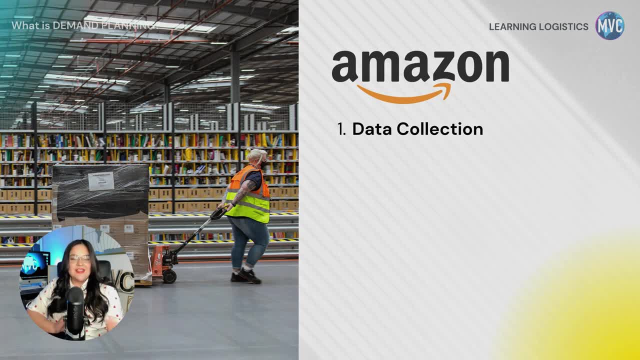 So all of this is data, is information. It's something that Amazon can use to better serve you as a customer. Some may find it creepy, but you know it's up for debate and that's another whole discussion. Amazon really does use this data to give you a better consumer experience. all right, 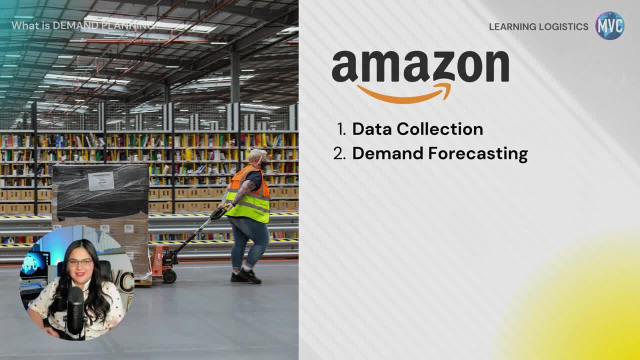 Next in their step is demand forecasting. Now, based on the data collected, Amazon uses various statistical methods, models and forecasting techniques to estimate future demand for each product. This involves analyzing historical sales pattern, seasonal fluctuations and other factors that can impact demand. 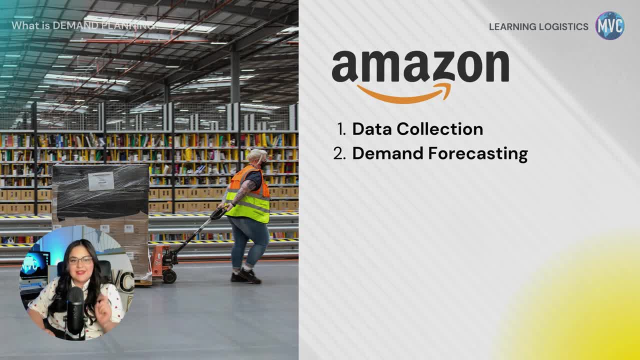 Amazon also considers external factors such as economic conditions, consumer behavior and competitor activity when forecasting for demand. Next is, or third is, inventory planning. Once the demand forecast has been determined, Amazon uses this information to plan inventory levels for each product. 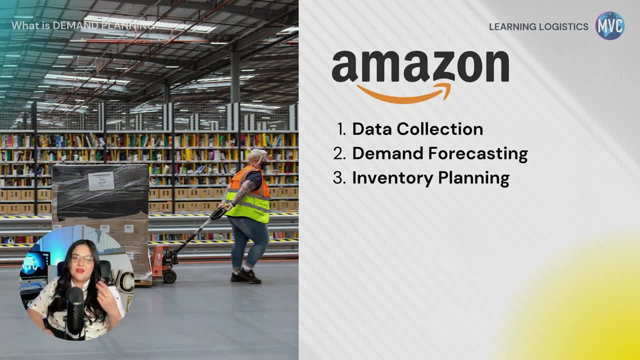 This involves setting safety stocks levels, reorder points and lead times to ensure their products are always available when customers need them. Amazon also uses demand sensing techniques to adjust inventory levels in real time based on actual demand. It's important to keep in mind that inventory levels are very important for customer demand. 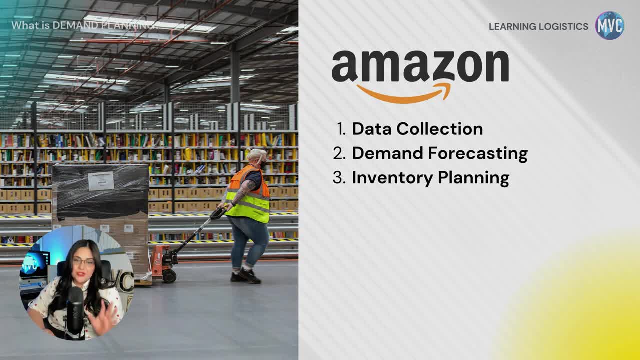 They have the ability to do this. Your system is very sophisticated in order to be able to do this in real time. Next, we have supplier collaboration. Amazon works closely with its suppliers to ensure that they can meet the demand for each product. This involves sharing the demand forecasts, inventory levels. 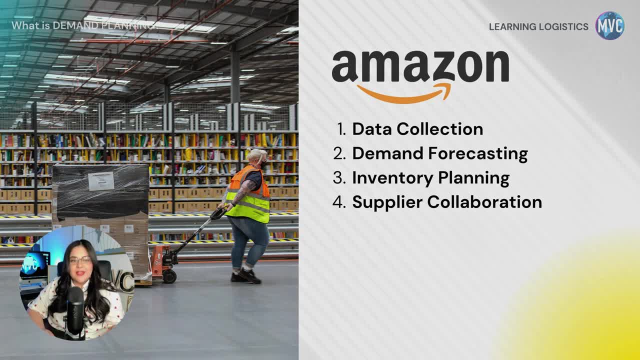 and production schedules with suppliers to help them plan their operations accordingly. Amazon also uses what is known as a Vendor-Managed Inventory Schedule, which is a vendor-managed inventory schedule. Vendor-Managed Inventory Schedule allows suppliers to manage inventory levels on behalf of Amazon. 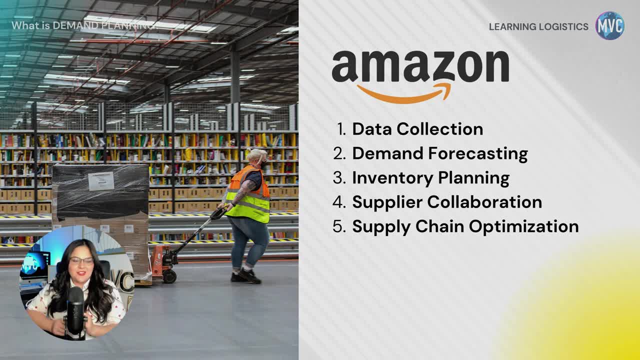 Next, we have Supply Chain Optimization. Amazon continuously optimizes its supply chain to ensure that products are delivered to customers in a timely and cost-effective manner. This involves using advanced logistics algorithms and transportation management systems to optimize delivery routes, reduce transportation costs and to minimize the lead time. 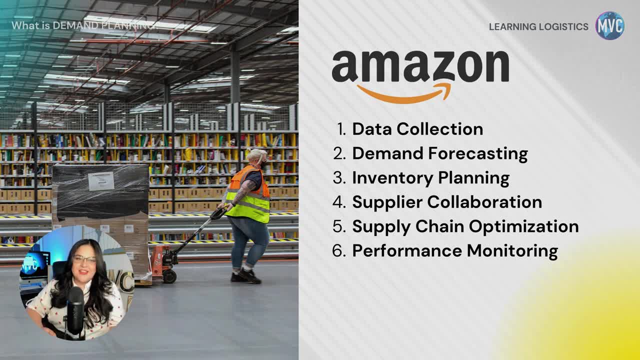 And finally, we have Performance Monitoring. Amazon closely monitors the performance of its supply planning process to ensure that it's meeting its objectives. This involves tracking key performance metrics such as forecast accuracy, inventory turnover and customer satisfaction. Amazon uses this information to identify areas for improvement. 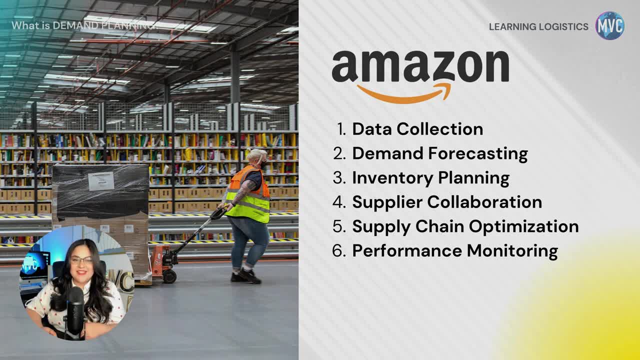 and to make changes to the demand planning process as needed. Now, overall, as you can see from these steps or this process that Amazon has, the demand planning process is really complex and a very sophisticated system that allows them to meet the ever-changing demands of their customers. 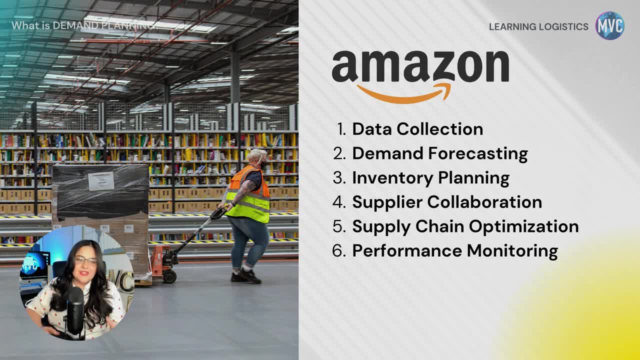 By using advanced analytics, machine learning and supply chain optimization techniques, Amazon really is able to forecast demand accurately, Plan inventory levels effectively and optimize their supply chain to deliver products to customers. Now, the next example I have for you is Zara, the fast fashion retailer. 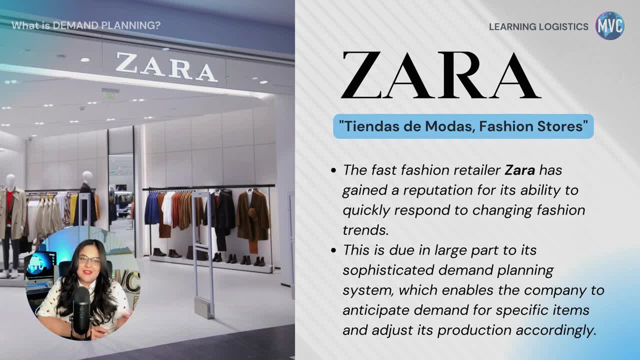 Now Zara has gained a reputation for its ability to quickly respond to the changing fashion trends, and they sort of started the trend of fast fashion that we see replicated in many other businesses and companies nowadays. Now, this is due in large part to their sophisticated demand planning system. 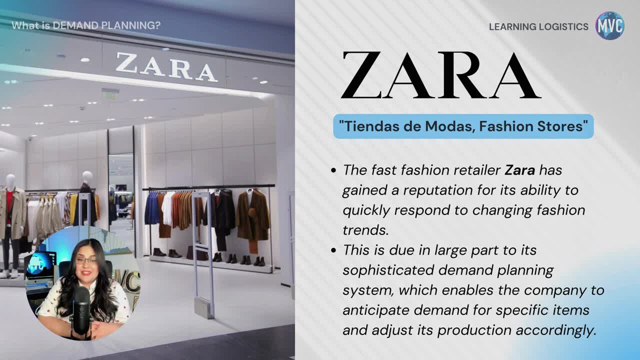 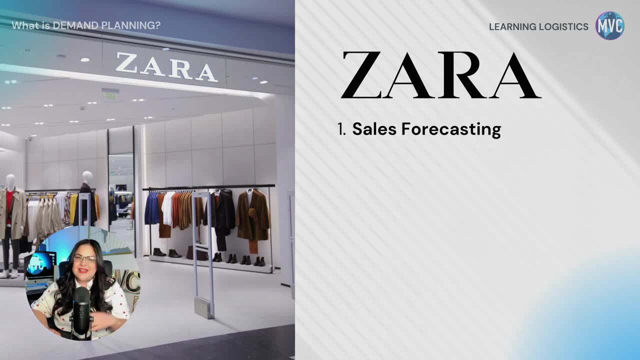 which enables the company to anticipate demand for specific items and adjust its production accordingly. Zara, like other fashion retailers, relies on demand planning to ensure they have enough inventory to meet customer demand, while minimizing waste and overstock. Here I'm going to take you through the step-by-step overview. 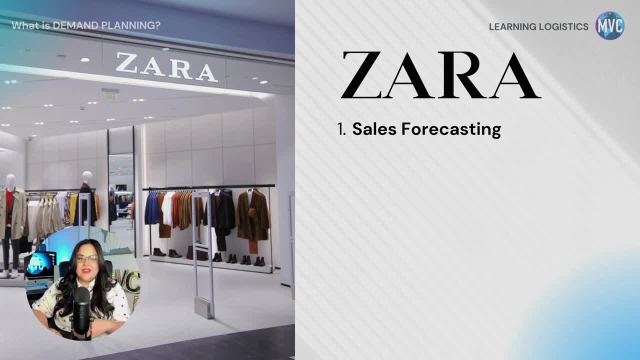 of what Zara's demand planning process looks like. First up, we have sales forecasting. Zara's demand planning process starts with sales forecasting. The sales team provides input on historical data or historical sales data, current sales trends and expected market conditions. 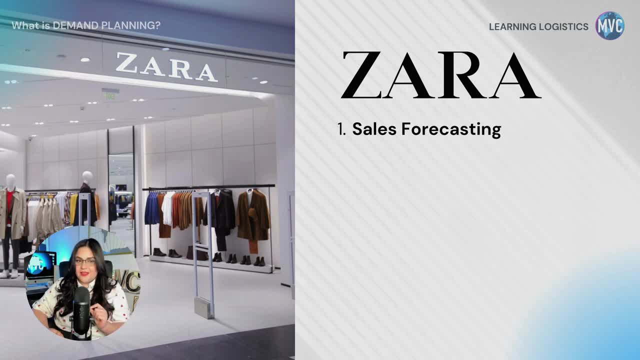 to predict future demand for each product category. This helps Zara understand how much stock they will need to produce and allocate to each of their stores. Next, we have inventory analysis. Zara then conducts an inventory analysis to determine how much stock they currently have on hand and where it is located. 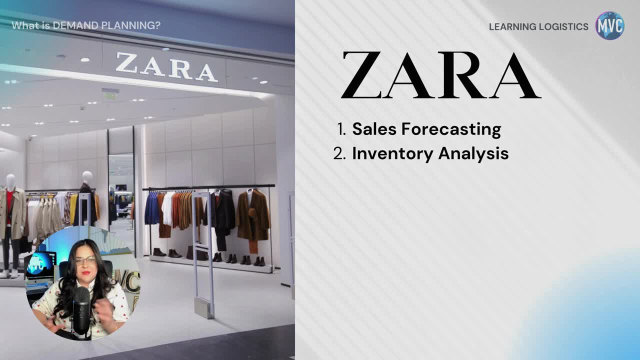 This helps them decide how much new stock needs to be produced and shipped to each store to meet the forecasted demand. So the third step is design and production. planning Was demand has been forecasted And inventory has been analyzed, Zara's design and production team work together to plan. 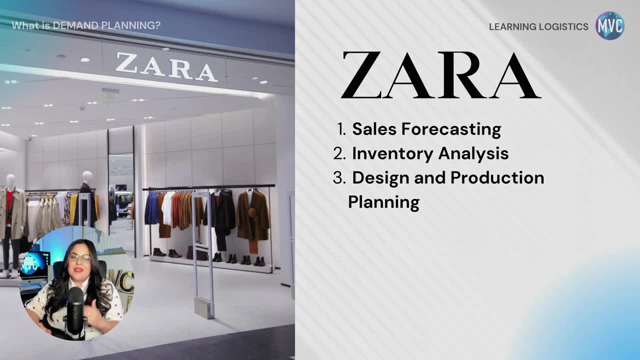 when new products will be produced and when This process includes setting timelines for each stage of production, from sourcing raw materials to finalizing designs, to manufacturing and shipping finished products. Next is allocation planning. Zara then uses the sales forecast and the inventory analysis to determine how much inventory should be allocated to each store. 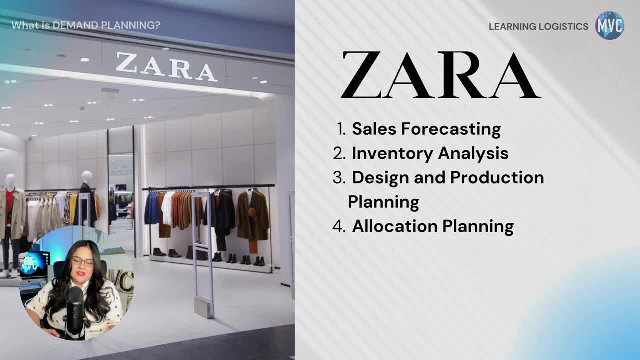 This is based on factors like past historical sales performance, store location and the demographics of the area the store is located in. The final step is review and adjust Throughout the season. Zara continuously reviews and adjusts their demand planning process based on actual sales performance. 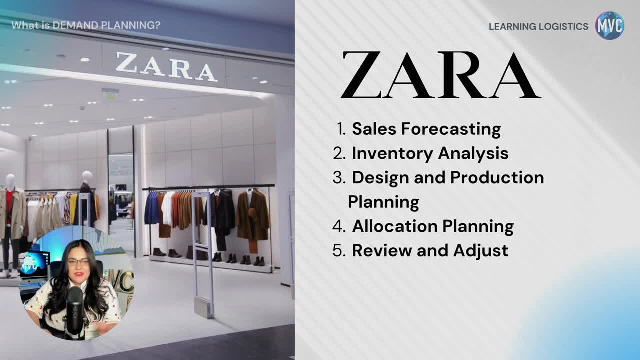 and inventory status. This allows them to quickly respond to changes in consumer demand and adjust production and allocation accordingly. Overall, Zara's demand planning process is a continuous cycle of forecasting, analysis and planning, as well as adjustment. All of this and everything that they do is really aimed at ensuring 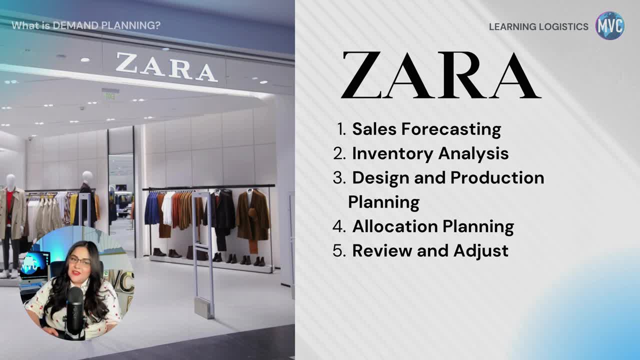 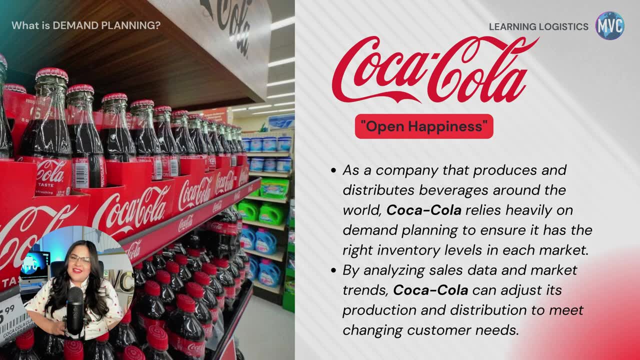 that the right products are available in the right quantities at the right stores to meet customer demand. And the last example that I have for you is Coca-Cola. As a company that produces and distributes its beverages around the world, Coca-Cola relies heavily on demand planning. 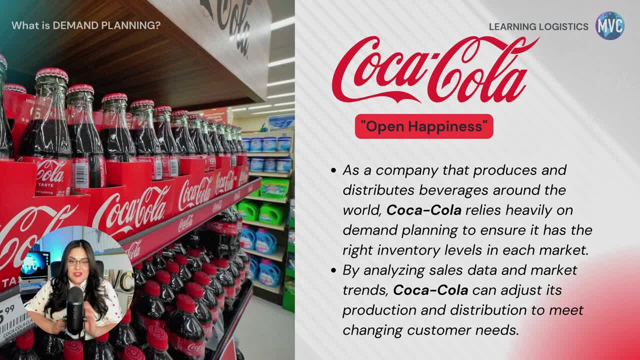 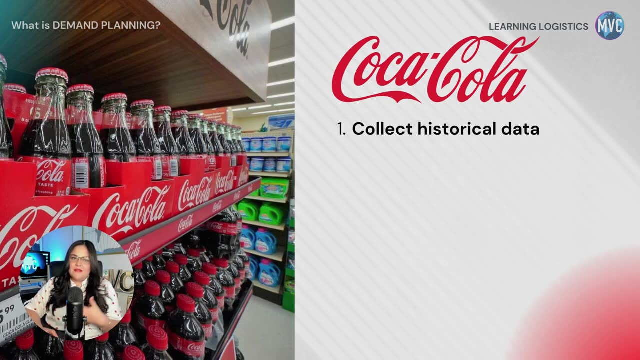 to ensure it has the right inventory levels in each of the markets that they serve. By analyzing sales data and market trends, Coca-Cola can adjust its production and distribution to meet the changing customer needs. So here we're going to talk about the steps that Coca-Cola typically follows. 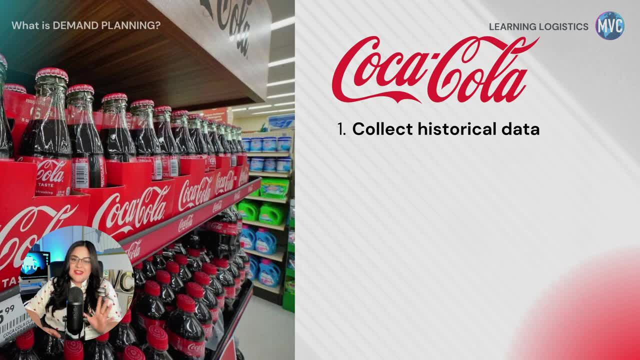 in their demand planning process. The first one is to collect historical data. The first step here will be for Coca-Cola's demand planning process, or demand planning team- is to collect historical data on sales, production and other key metrics. This data is typically collected from a variety of sources. 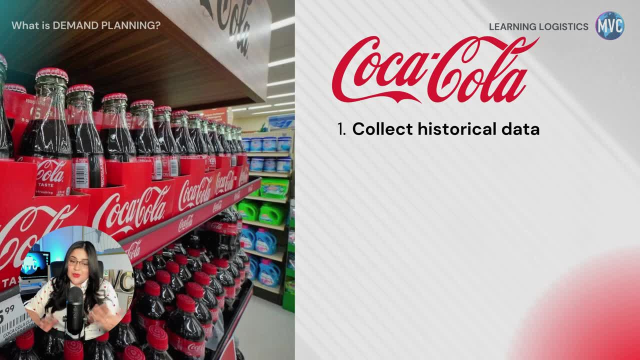 including POS or points of sale systems, distributors and retailers. Step two is clean and normalize the data. You'll hear this a lot in demand planning. Once the data has been collected, it is cleaned and normalized to ensure that it is accurate and consistent. 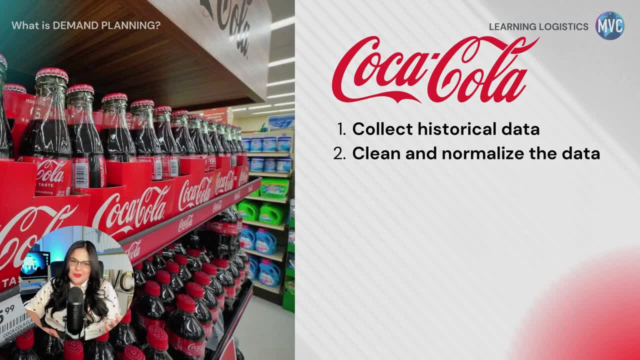 This involves basically removing any errors, any duplicates or outliers from the data set. The next step is to analyze the data to identify any trends, patterns or other insight that can be used to inform the demand planning process or team. This analysis may involve using statistical models. 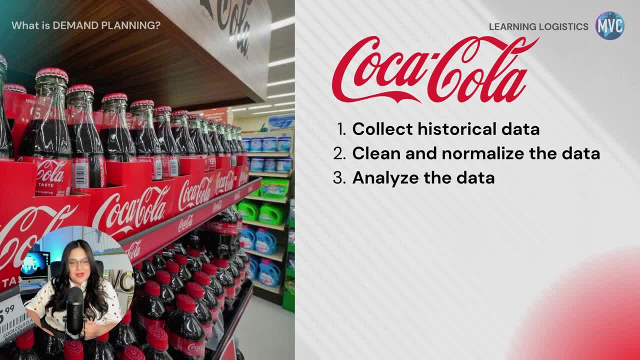 or other techniques to forecast demand based on historical trends. The next step is to collaborate with stakeholders Once the data has been analyzed. Coca-Cola's demand planning team works closely with stakeholders across the organization to gather input and insights into demand drivers, market trends and other factors that may impact the demand. 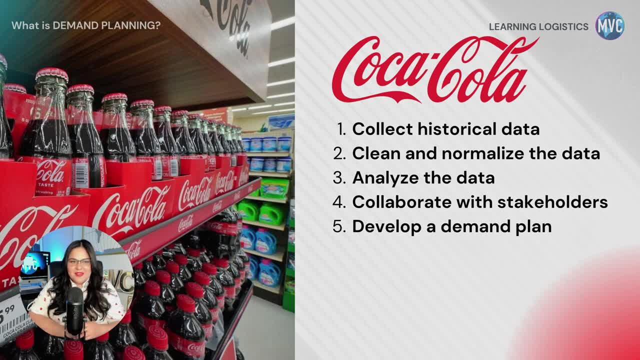 Next, we have to develop a demand plan. Based on the insights gathered from the data analysis and from the stakeholder collaboration, Coca-Cola's demand planning team develops the demand plan. This plan outlines projected sales volume. projected sales volumes, production schedules. 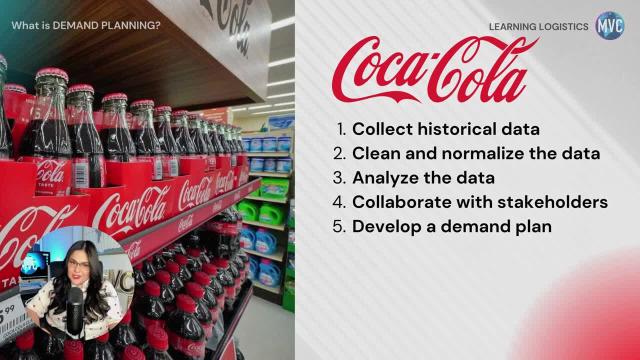 and the inventory levels for each product in each market. The next step for Coca-Cola is to review and refine the plan. The demand plan will be reviewed and refined based on the feedback from stakeholders and any new information or insights that may have emerged since the demand was initially developed. 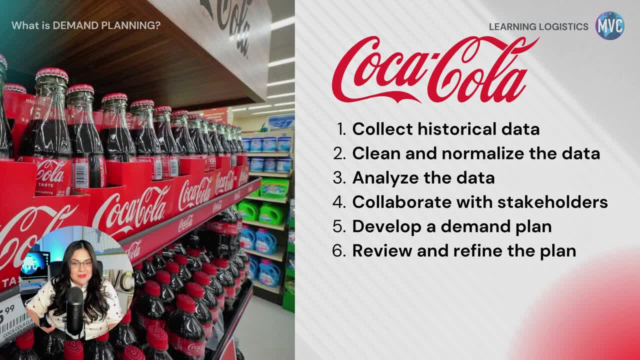 This is a great example of being flexible and being agile enough so that you can make tweaks and changes and refine the plan that was already established. as we mentioned earlier, Step number seven is to monitor performance Once the demand plan has been finalized. Coca-Cola's demand planning team closely monitors performance. to ensure that the actual sales and the production volumes align with the projected plan. Any variances, or then changes, can be analyzed and the demand plan may be adjusted as needed to ensure that it remains aligned with the actual demand. And the last step is continuously improving the process. 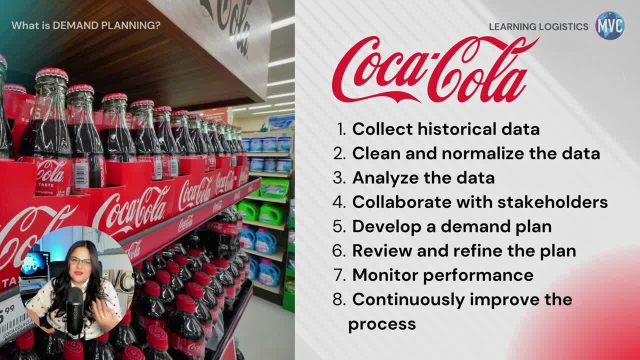 Coca-Cola's demand planning team continuously reviews and improves its demand planning process to ensure that it remains effective and efficient. This may involve implementing new tools or technologies, refining the forecasting models or making other improvements as needed. Overall, you can see that Coca-Cola's demand planning process 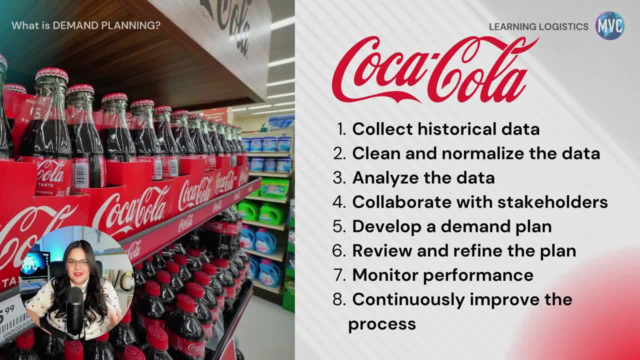 is complex and the process really involves data collection, analysis, stakeholder collaboration and also, like an ongoing performance monitoring and improvement, which always speaks volumes for the company and how they run things. By following these steps, Coca-Cola is able to effectively forecast demand. 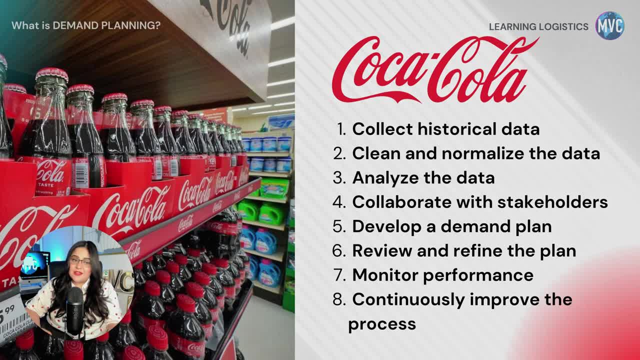 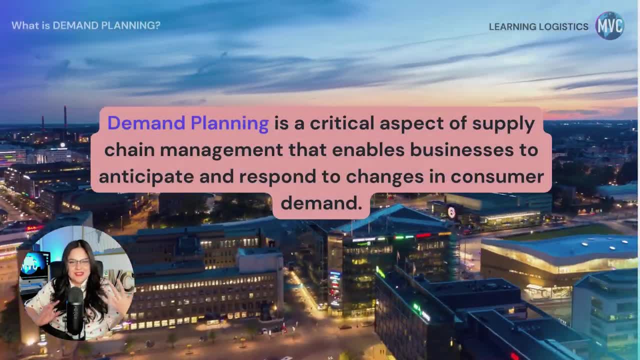 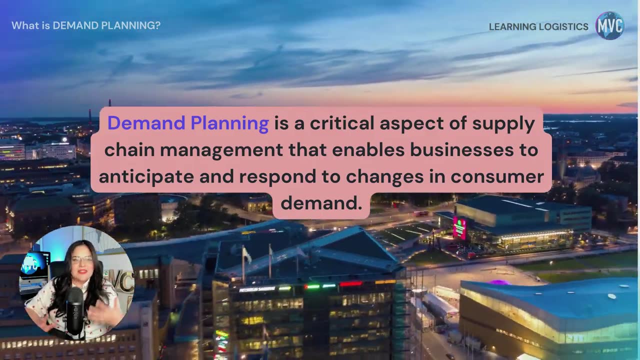 and ensure that it has the right inventory levels and production schedules in place to meet the customer's needs. Well, I hope you really enjoy some of those examples as far as what companies and what their demand planning process looks like, But I do want to make a very important point. 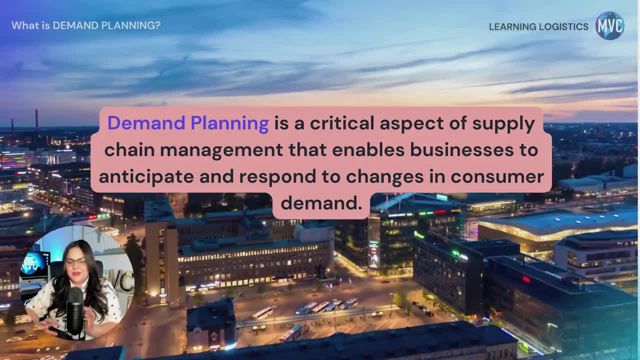 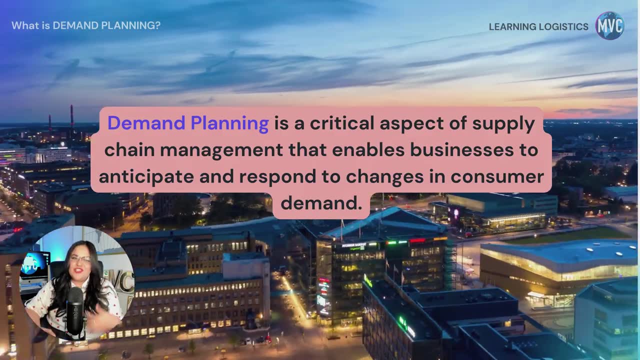 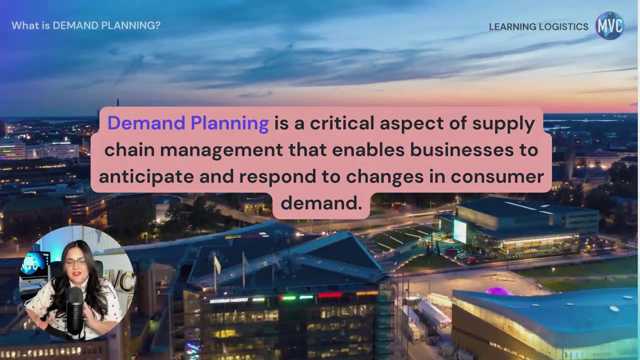 that demand planning is a critical aspect of supply chain management that enables businesses like Amazon, like Zara, like Coca-Cola and others to anticipate and respond to changes in consumer demand. By implementing effective demand planning strategies, processes, businesses can really help themselves to optimize their inventory levels. 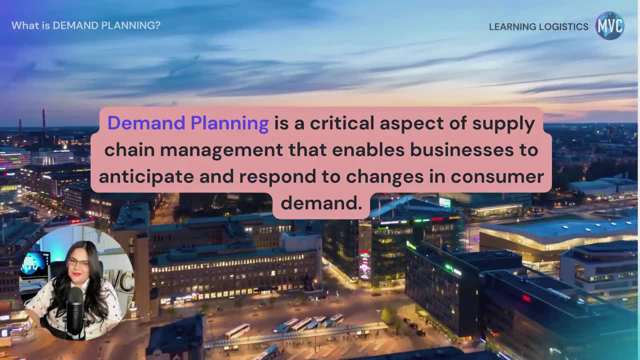 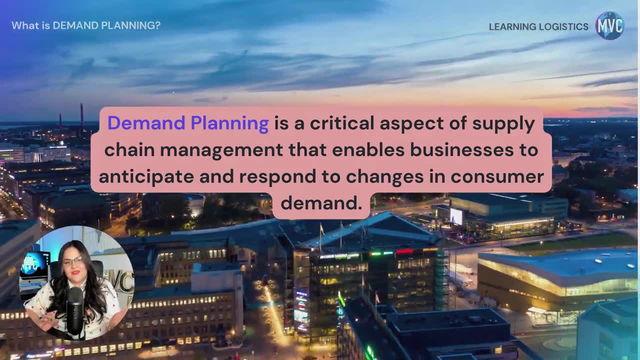 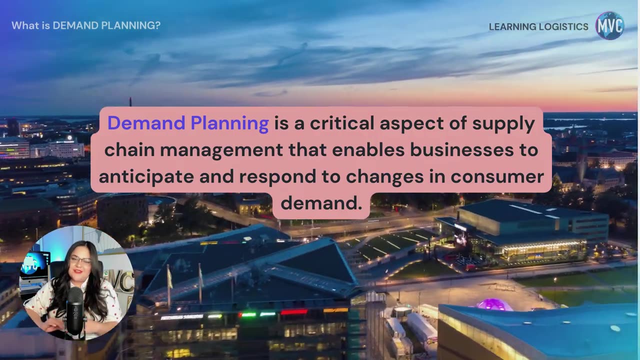 to reduce waste and to improve their bottom line. By accurately predicting future demand, businesses can really ensure that they have the right amount of inventory on hand to meet customers without the need to overstock or understock or sell out or stock out. 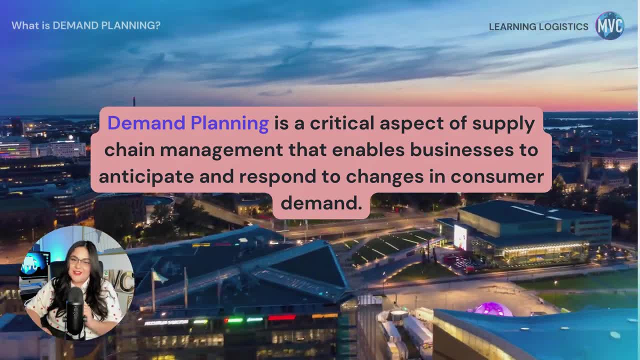 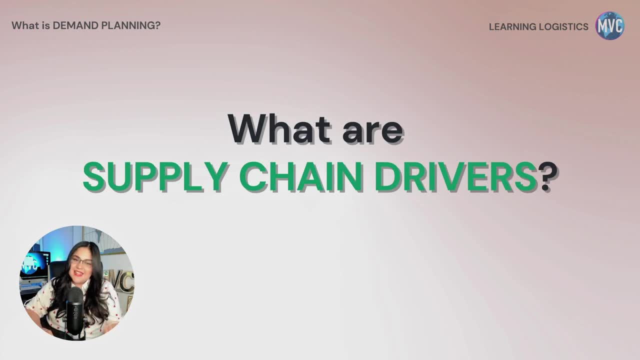 All right, so that's very important to know. So I hope you really learned a lot about demand planning in today's lesson. In the next lesson in the series, I will discuss what are supply chain drivers, So I hope you stay tuned for that. 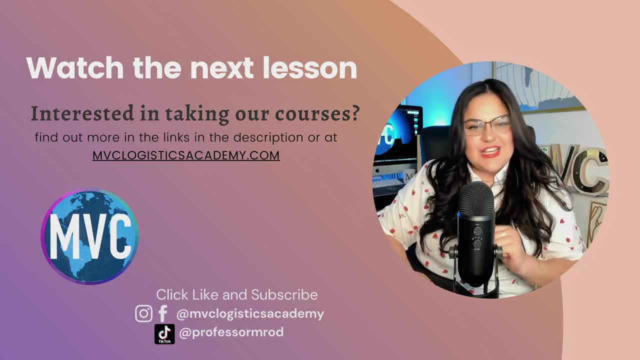 That is, though, the end of today's lesson, Lesson number eight, on what is demand planning. I thank you very much for watching. I hope you're finding this useful and informative and you're learning more and more about supply chain management with each video and each lesson.